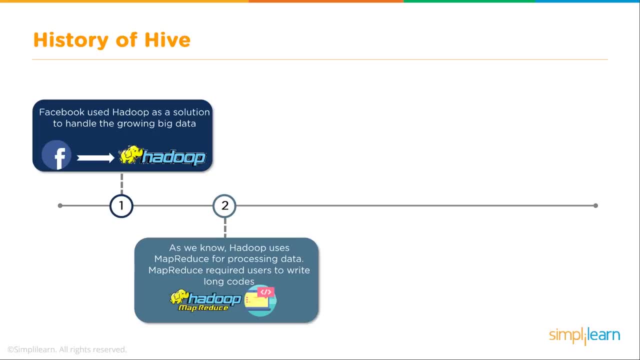 codes, And so you'd have these really extensive Java codes, very complicated for the average person to use. Not all users reversed in Java and other coding languages. This proved to be a disadvantage for them. Users were comfortable with writing queries in SQL. SQL has been around. 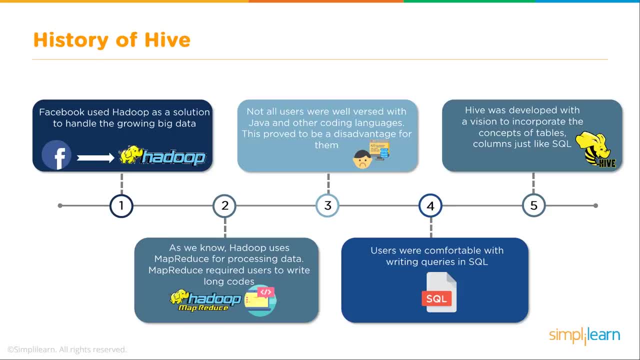 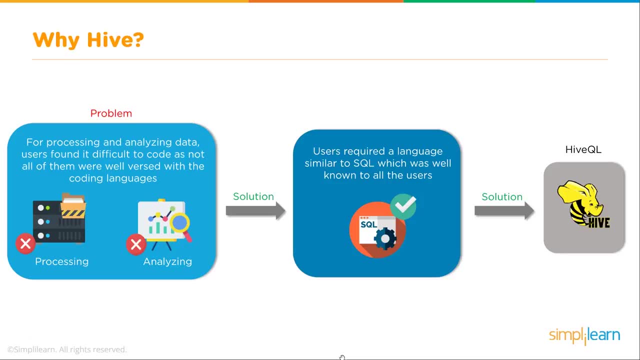 for a long time, but it's not a very long time, And so Hive was developed with the vision to incorporate the concepts of tables, columns, just like SQL. So why Hive? Well, the problem was for processing and analyzing data. Users found it difficult to code, as not all of them were well. 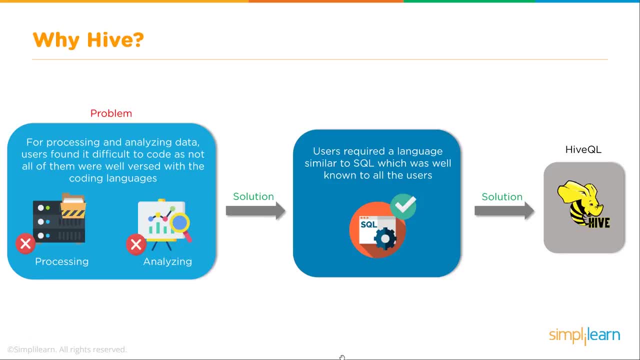 versed with the coding languages. You have your processing, you have your analyzing, And so the solution was required: a language similar to SQL, which was well known to all the users, And thus the Hive, or HQL, language evolved. What is Hive? 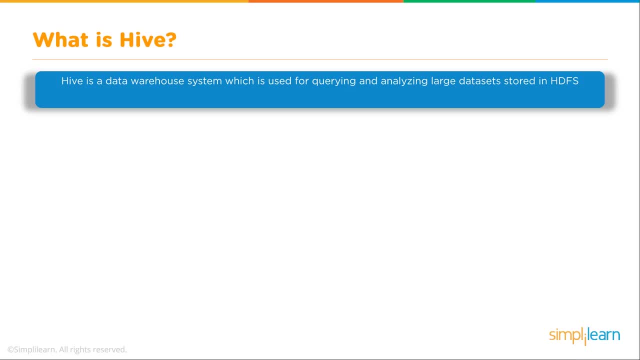 Hive is a data warehouse system which is used for querying and analyzing large data sets stored in the HDFS or the Hadoop file system. Hive uses a query language that we call HiveQL or HQL, which is similar to SQL. So if we take our user, the user sends out their Hive queries and then 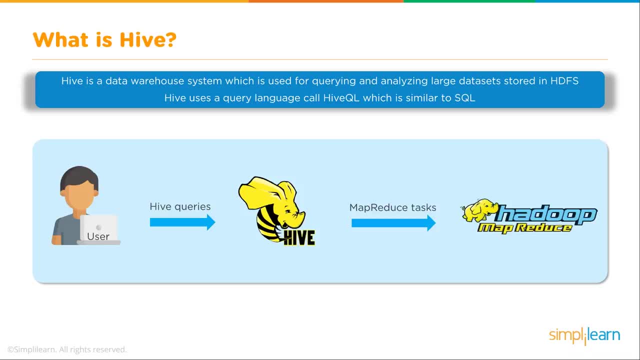 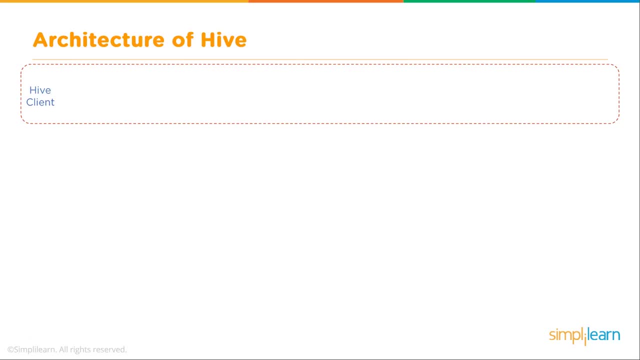 that is converted into a MapReduce tasks and then accesses the Hadoop MapReduce system. Let's take a look at the architecture of Hive. Architecture of Hive: We have the Hive client, So it could be the programmer, or maybe it's a manager who knows enough SQL to do a basic query. to look. 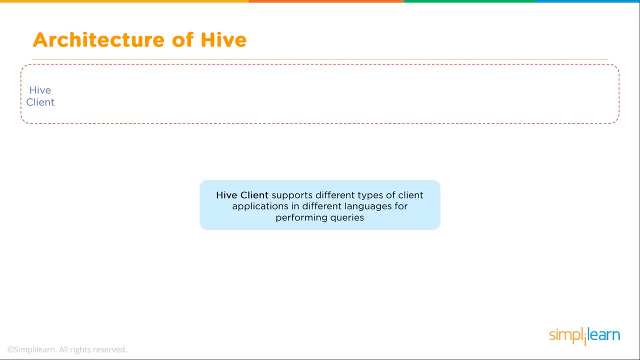 up the data they need. The Hive client supports different types of client applications in different languages for performing queries, And so we have our Thrift application and the Hive Thrift client. Thrift is a software framework. Hive server is based on Thrift so it can serve the 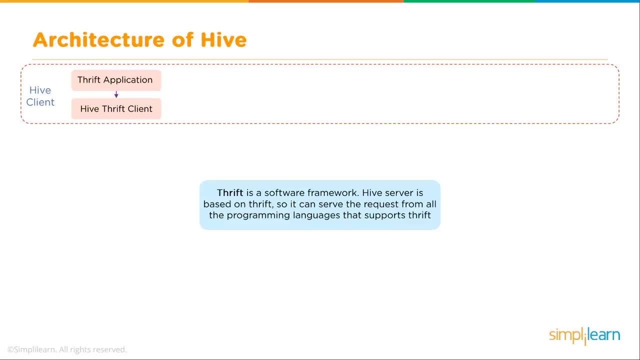 requests from all programming languages that support Thrift. And then we have our JDBC application and the Hive JDBC database. JDBC driver, JDBC Java database connectivity JDBC application is connected through the JDBC driver And then you have the ODBC application or the Hive ODBC driver, The ODBC or open database. 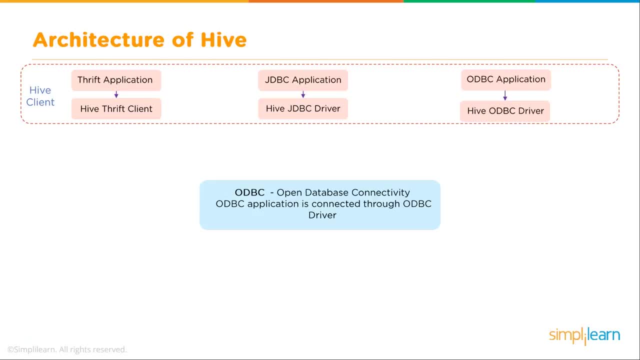 connectivity. The ODBC application is connected through the ODBC driver. With the growing development of all of our different scripting languages- Python, C++, Spark, Java- you can find just about any connection in any of the main scripting languages. So if you're using a, 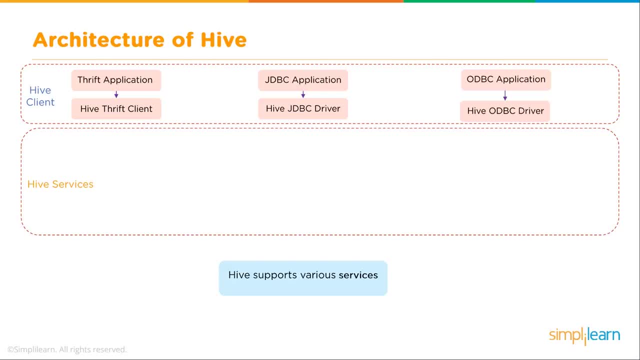 languages, and so we have our hive services. as we look at deeper into the architecture, hive supports various services, so you have your hive server, basically your thrift application or your hive thrift client, or your JDBC or your hive JDBC driver, your ODBC application or your hive ODBC driver. 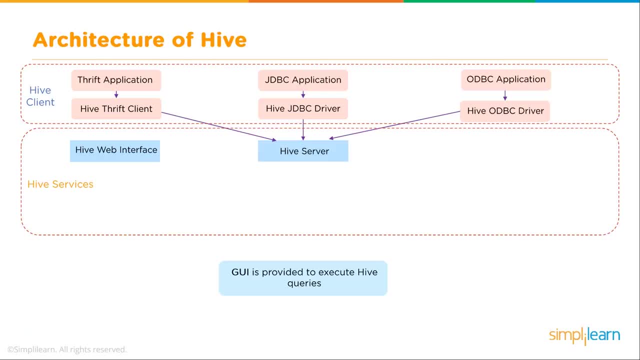 they all connect into the hive server and you have your hive web interface. you also have your CLI. now, the hive web interface is a GUI, is provided to execute hive queries and we'll actually be using that later on today so you can see kind of what that looks like and get a feel for what that means. commands are. 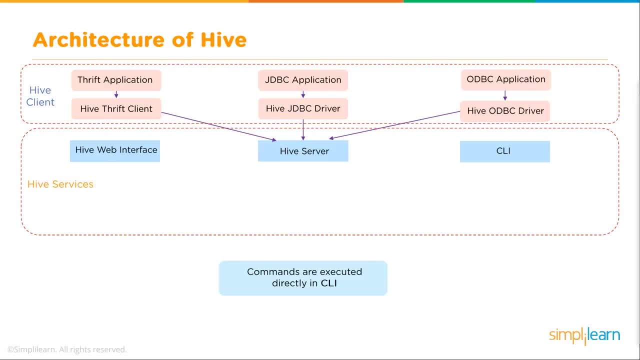 executed directly in CLI, and then the CLI is a direct terminal window, and I'll also show you that too, so you can see how those two different interfaces work. these then push the code into the hive driver. hive driver is responsible for all the queries submitted, so everything goes through that driver. let's take a. 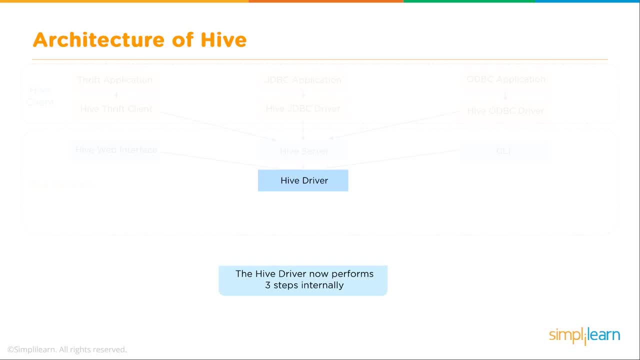 closer look at the hive driver. the hive driver now performed three steps internally. one is a compiler. hive driver passes query to compiler, where it is checked and analyzed. then the optimizer kicks in and the optimized logical plan in the form of a graph of MapReduce and HDFS tasks. 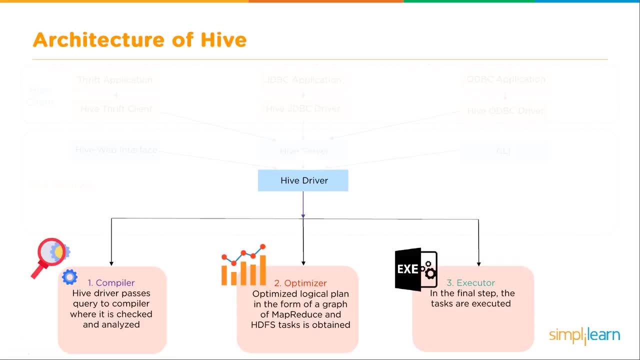 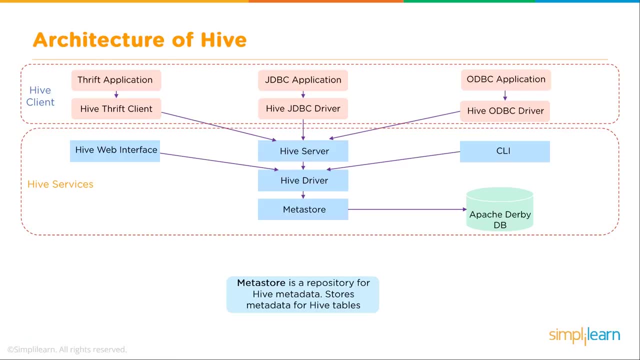 is obtained and then finally, in the executor, in the final step, the tasks are executed. we look at the architecture. we also have to note the meta store. meta store is a repository for hive metadata stores, metadata for hive tables, and you can think of this as your schema. and where is a? 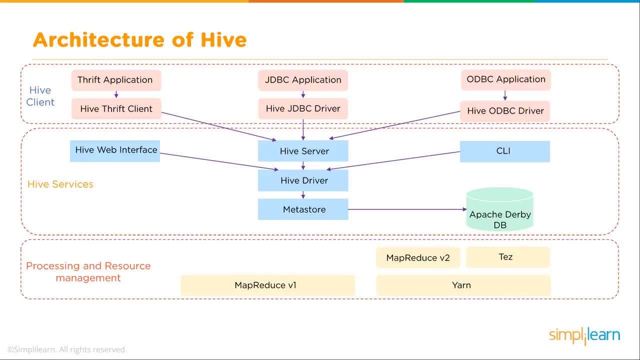 location and it's stored on the Apache Derby DB processing and resource management is all handled by the MapReduce v1. you'll see MapReduce v2, the yarn and the Tez. these are all different ways of managing these resources, depending on what version of Hadoop you're in. hive uses MapReduce framework. 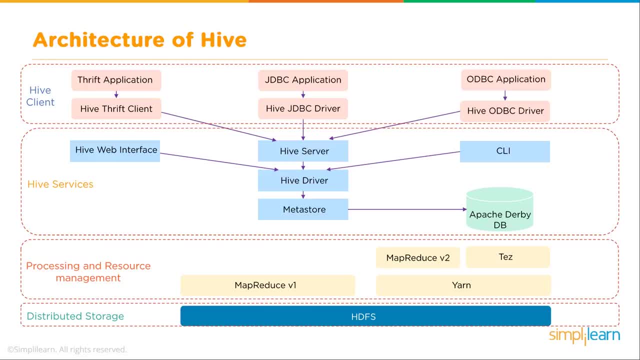 to process queries. and then we have our distributed storage, which is the HDFS, and if you looked at our Hadoop tutorials, you'll know that these are on commodity machines and are linearly scalable means they're very affordable. a lot of time when you're talking about big data. 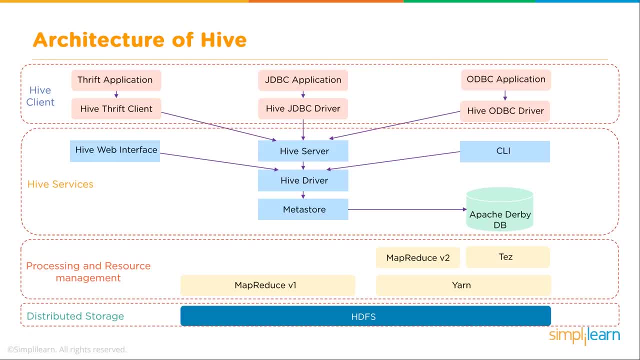 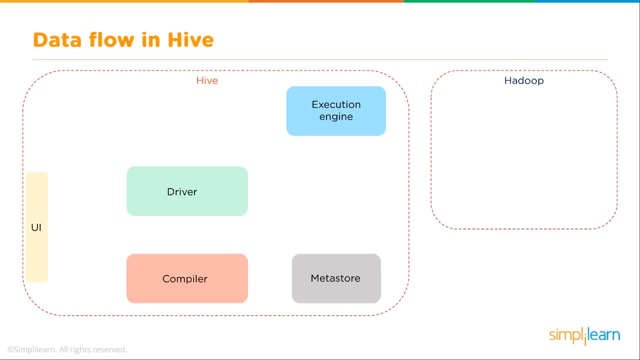 you're talking about a tenth of the price of storing it on enterprise computers. and then we look at the data flow in hive. so in our data flow in hive we have our hive in the Hadoop system and underneath the user interface or the UI we have our driver, our compiler, our execution engine and our meta store. that. 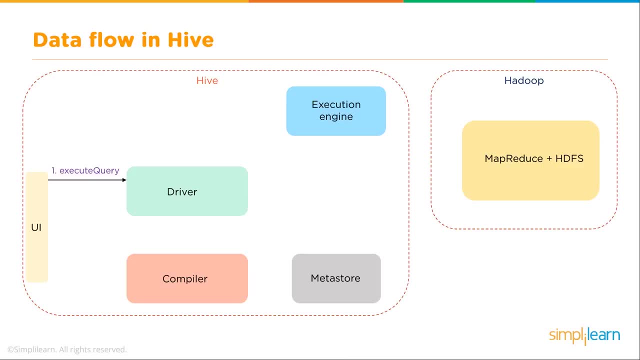 all goes into the MapReduce and the Hadoop file system. so when we execute a query, you see it coming in here. it goes into the driver. step one, step two, we get all the information in the machine. the timer what are we going to do? refers to: 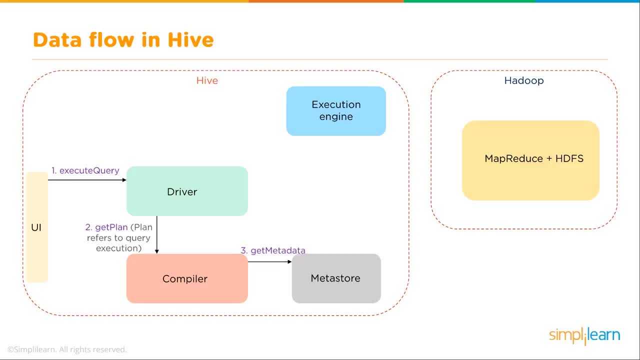 the query execution. then we go to the meta data. it's like: well, what kind of meta data are we actually looking at? where is this data located? what is the schema on it? then this: that comes back with the metadata into the compiler. then the compiler takes all that information and the send plan returns it to the 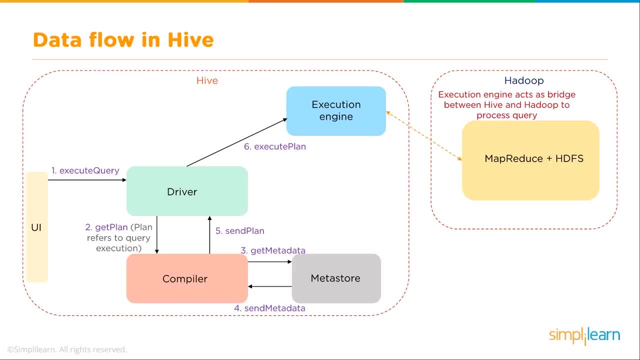 driver. the driver then sends the execute plan to the execution engine. once it's in the execution engine, the execution engine axe as a bridge between hive and And that's going into your MapReduce and your Hadoop file system or your HDFS. And then we come back with the metadata operations. 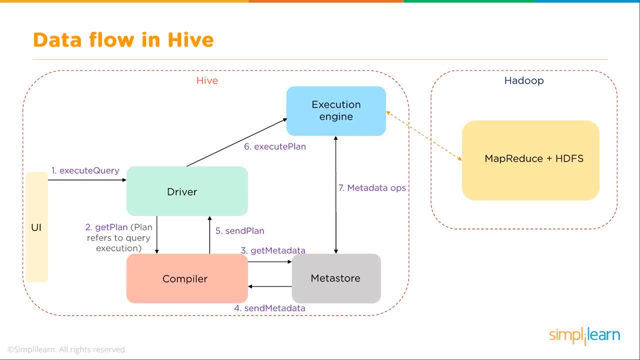 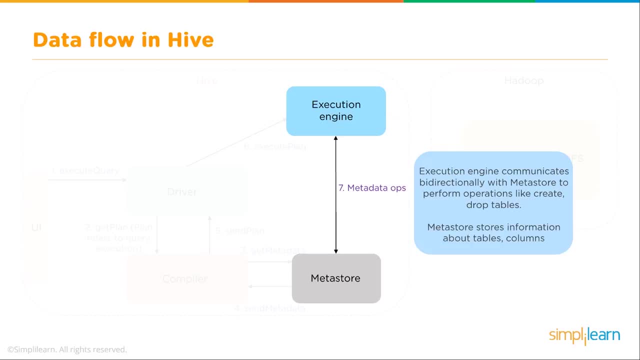 It goes back into the Metastore to update or let it know what's going on, which also goes to the communication between the execution engine and the Metastore. Execution engine communications is bidirectionally with the Metastore to perform operations like create drop tables. 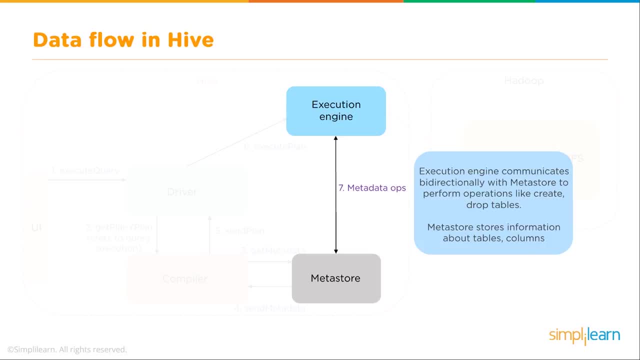 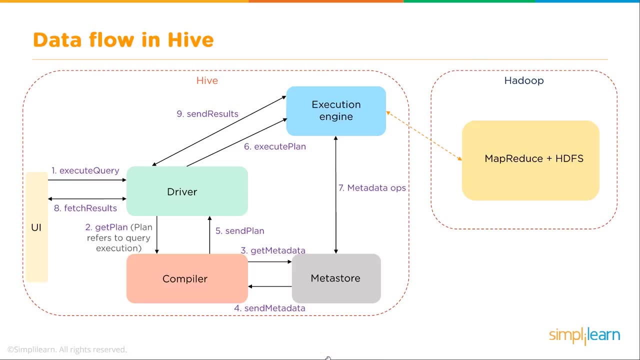 Metastore stores information about tables and columns. So again we're talking about the schema of your database And once we have that, we have a bidirectional send results communication back into the driver And then we have the fetch results which goes back to the client. 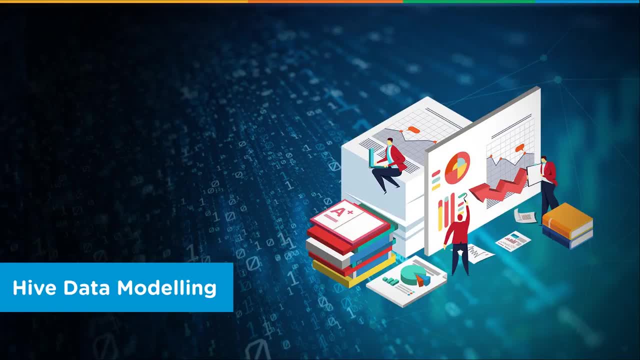 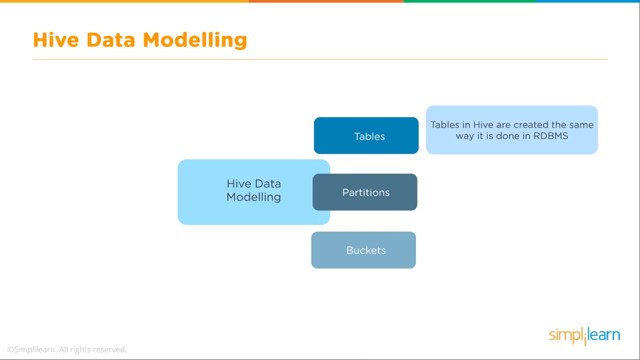 So let's take a little bit. look at the Hive data modeling. Hive data modeling: So you have your Hive data modeling, You have your tables, you have your partitions and you have buckets. The tables in Hive are created the same way it is done in RDBMS. 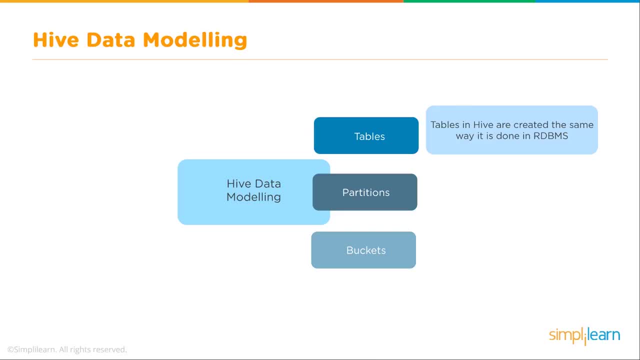 So when you're looking at your traditional SQL server or MySQL server, where you might have enterprise equipment and a lot of people pulling and moving stuff off of there, the tables are going to look very similar And this makes it very easy to take that information. 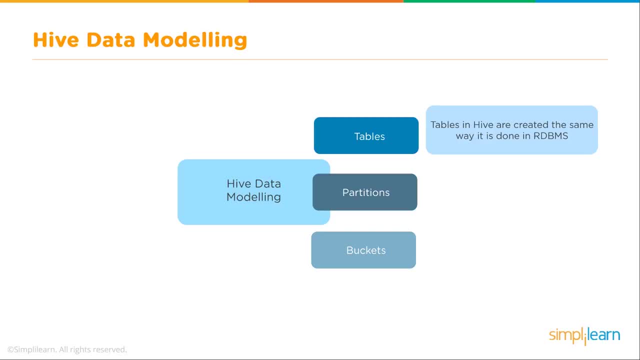 and let's say you need to keep current information but you need to store all of your years of transactions back into the Hadoop Hive So you match those. Those all kind of look the same, The tables are the same, Your databases look very similar and you can easily import them back. 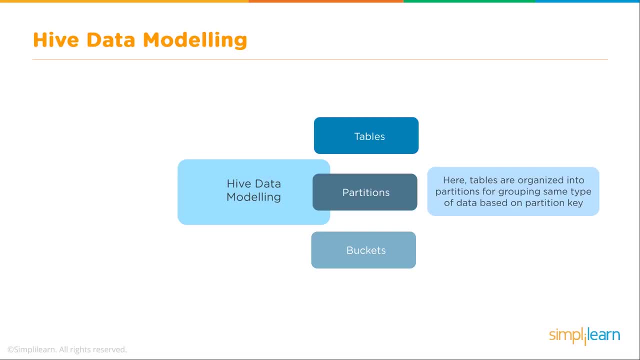 You can easily store them into the Hive system. Partitions: Here tables are organized into partitions for grouping same type of data based on partition key. This can become very important for speeding up the process of doing queries. So if you're looking at dates as far as like your employment dates of employees, 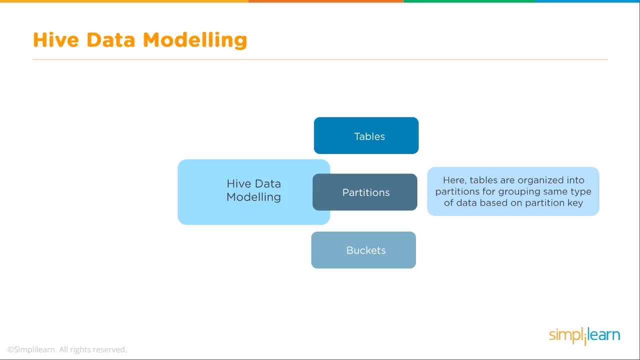 if that's what you're tracking, you might add a partition there, because that might be one of the key things that you're always looking up as far as employees are concerned. And finally, we have buckets. Data present in partitions can be further divided into buckets for efficient querying. 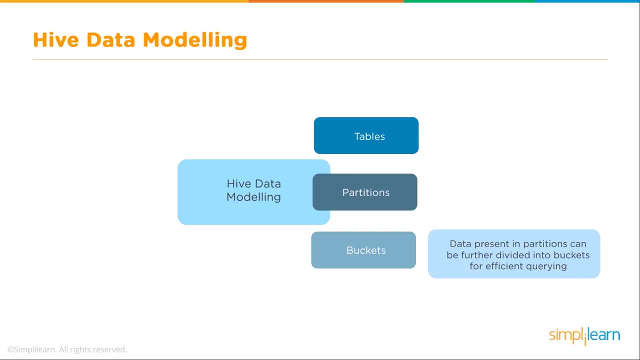 Again, there's that Efficiency At this level. a lot of times you're working with the programmer and the admin of your Hadoop file system to maximize the efficiency of that file system. So it's usually a two-person job and we're talking about Hive data modeling. 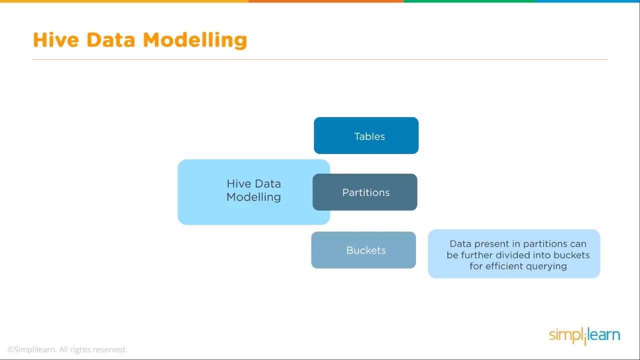 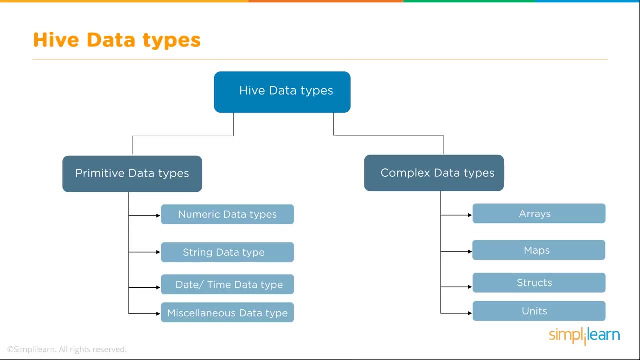 You want to make sure that they work together and you're maximizing your resources. Hive data types. So we're talking about Hive data types. We have our primitive data types and our complex data types. A lot of this will look familiar. It mirrors a lot of stuff in SQL. 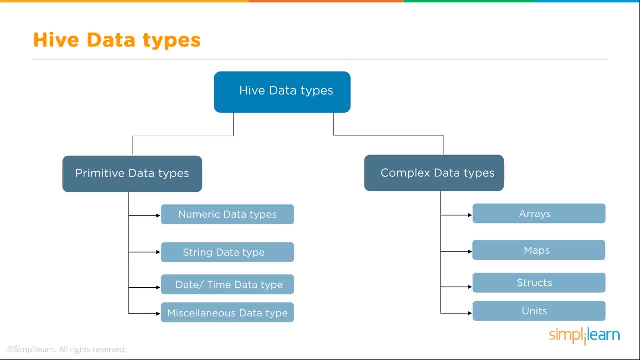 In our primitive data types we have the numerical data types, string data type, date-time data type and miscellaneous data type, And these should be very. they're kind of self-explanatory, but just in case. Numerical data is your floats, your integers, your short integers. 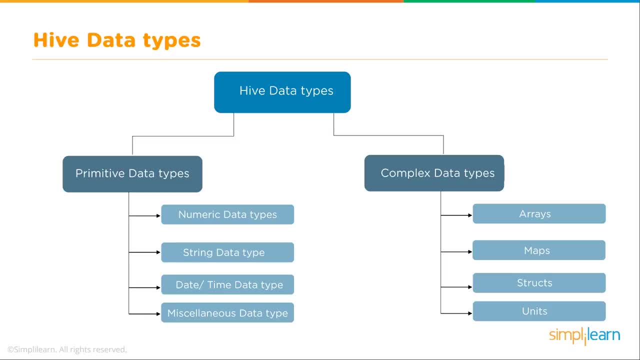 All of that numerical data comes in as a number. A string of course is characters and numbers, And then you have your date-time stamp And then we have kind of a general way of pooling your own created data types. And that's our miscellaneous data type. 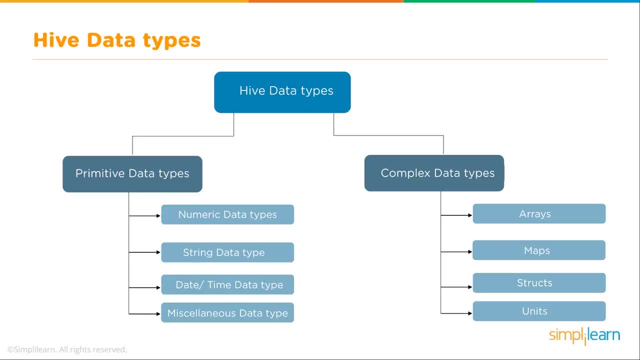 And we have complex data types. So you can store arrays, you can store maps, you can store structures and even units in there As we dig into Hive data types and we have the primitive data types and the complex data types. So we look at primitive data types and we're looking at numeric data types. 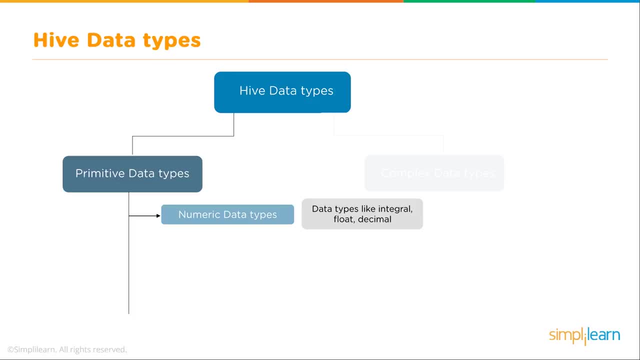 Data types like an integer, a float, a decimal. those are all stored as numbers in the Hive data system. A string data type Data types like characters and strings. You store the name of the person you're working with, John Doe. the city: Memphis. the state: Tennessee, maybe it's Boulder, Colorado, USA, or maybe it's Hyperbad, India. 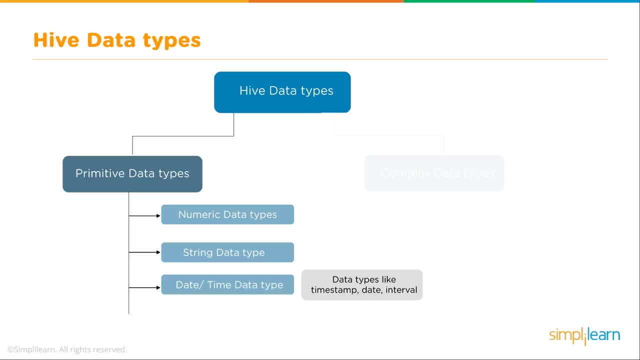 That's all going to be string. It's stored as a string character And, of course, we have our date-time data type, Data types like timestamp, date interval. those are very common as far as tracking sales, anything like that. 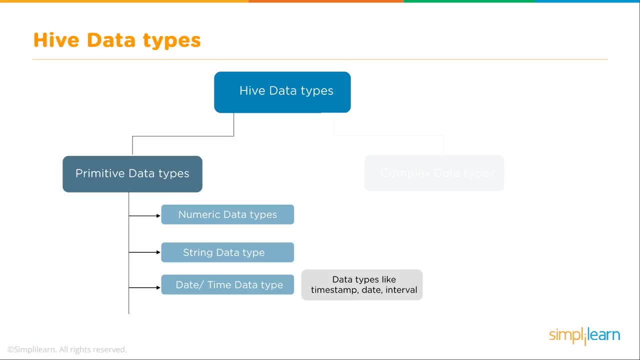 So you can just think if you can type a stamp of time on it, or maybe you're dealing with a race and you want to know the interval- how long did the person take to complete whatever task it was? All of that is date-time data type. 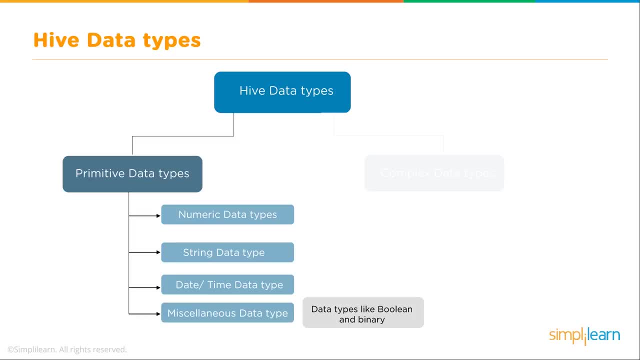 And then we talk miscellaneous data type. These are like Boolean and binary, And when you get into Boolean and binary, you can actually almost create anything in there but your yes-no's, 0, 1.. Now let's take a look at complex data types a little closer. 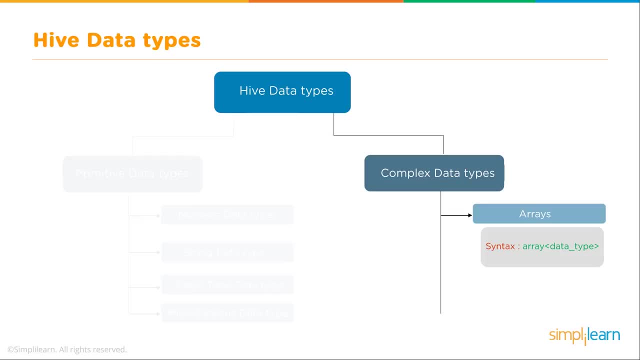 We have arrays, So your syntax is of data type and it's an array And you can just think of an array as a collection of same entities- 1,, 2,, 3,, 4,- and you can just call it a set of numbers. 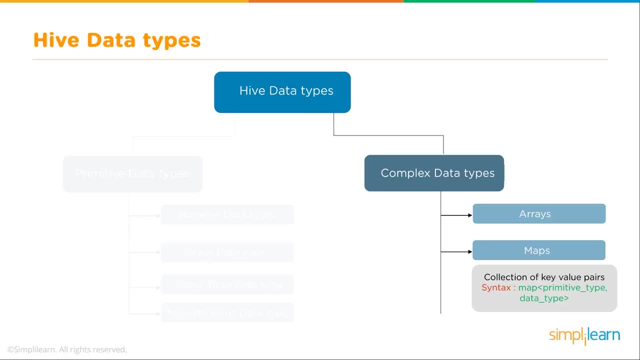 And you have maps. This is a collection of key-value pairs, So understanding maps is so central to Hadoop. So when we store maps, you have a key which is a set. You can only have one key per mapped value. And so in Hadoop, of course, you collect the same keys and you can add them all up or do something with all the contents of the same key. 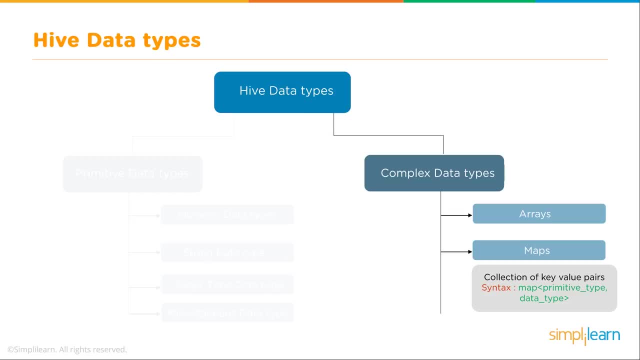 But this is our map as a primitive type, data type in our collection of key-value pairs And then collection of complex data with comment. So we can do this. We can have a structure. We have a column name, data type, comment, column comment. 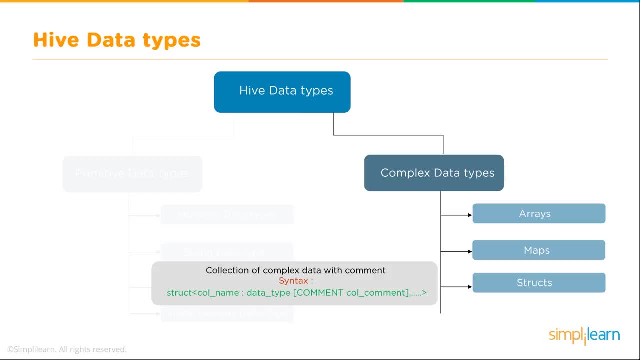 So you can get very complicated structures in here with your collection of data and your commented setup. And then we have units, And this is a collection of heterogeneous data types. So the syntax for this is union type, data type, data type and so on. 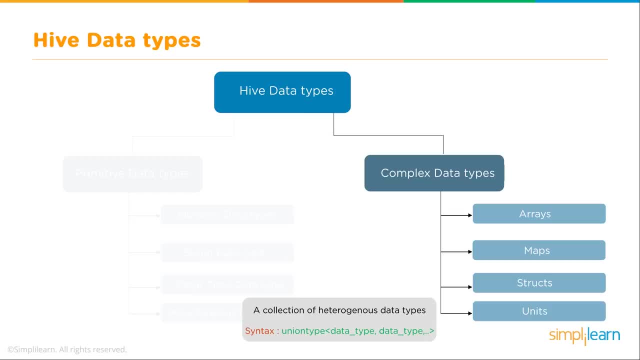 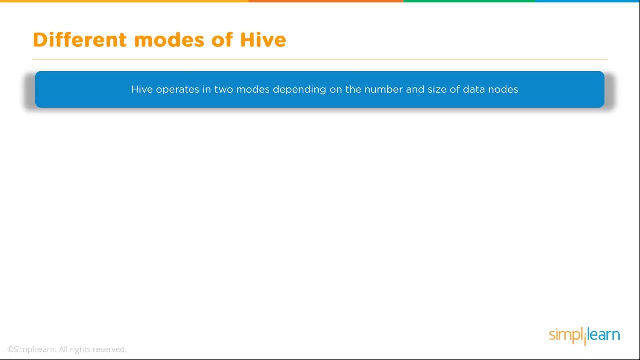 So it's all going to be the same, A little bit different than the arrays, where you can actually mix and match Different modes of Hive. Hive operates in two modes, depending on the number and size of data nodes. We have our local mode and our map reduce mode. 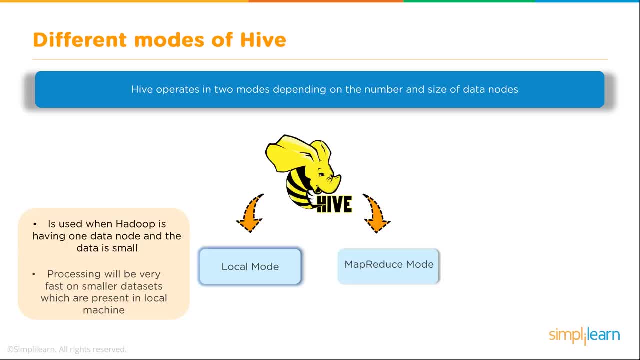 When we talk about the local mode, it is used when Hadoop is having one data node and the data is small. Processing will be very fast on the smaller data sets which are present in local machine. And this might be that you have a local file of stuff you're uploading into the Hive and you need to do some processes in there. 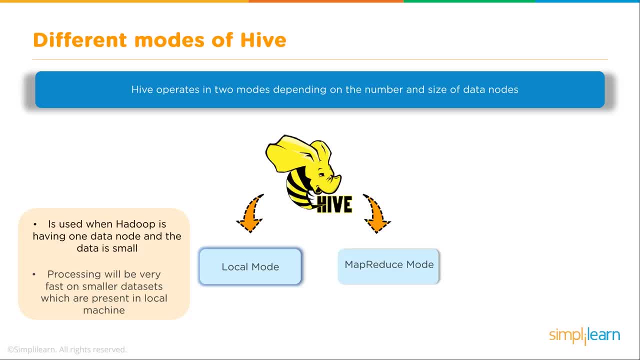 You can go ahead and run those Hive processes and queries on it. Usually you don't see much in the way of a single node Hadoop system. If you're going to do that, you might as well just use an Hive. You might as well just use an SQL database or even a Java SQLite or something. 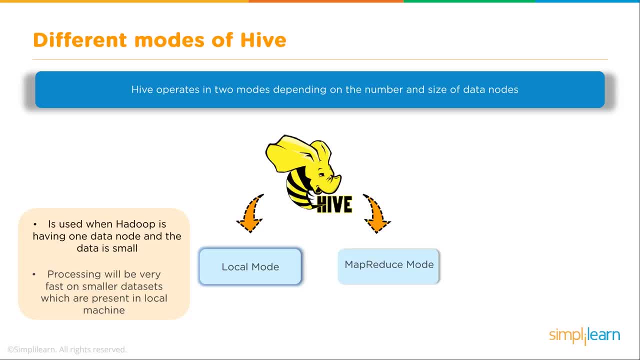 Python is SQLite, So you don't really see a lot of single node Hadoop databases. But you do see the local mode in Hive where you're working with a small amount of data that's going to be integrated into the larger database, And then we have the map reduce mode. 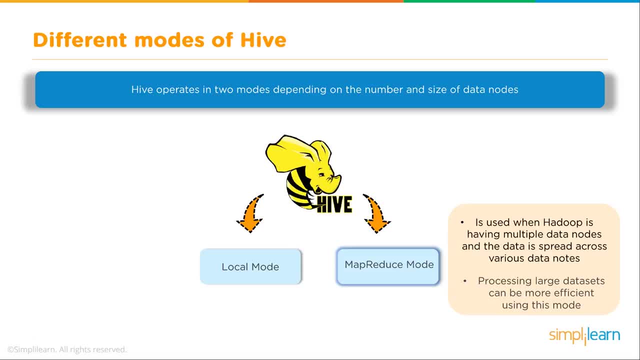 This is used when Hadoop is having multiple data nodes and the data is spread across various data nodes. Processing large data sets can be more efficient using this mode, And this you can think of: instead of it being one, two, three or even five computers, we're usually talking with a Hadoop file system. 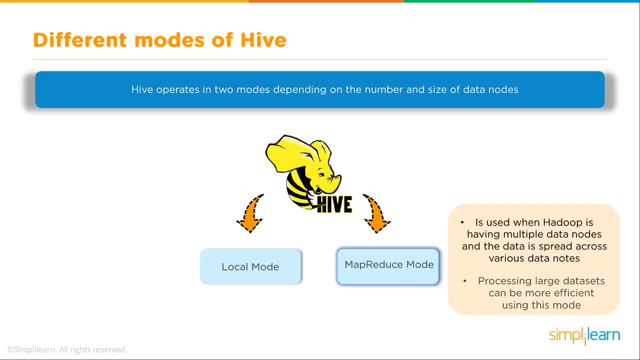 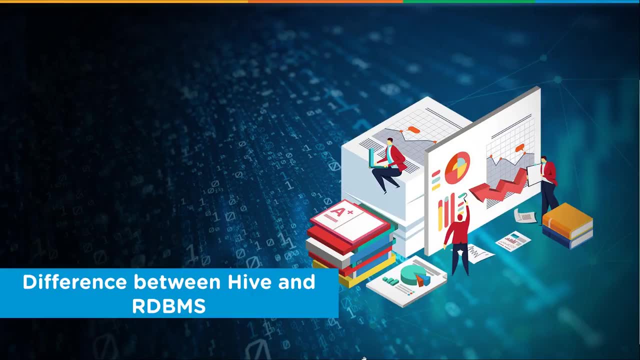 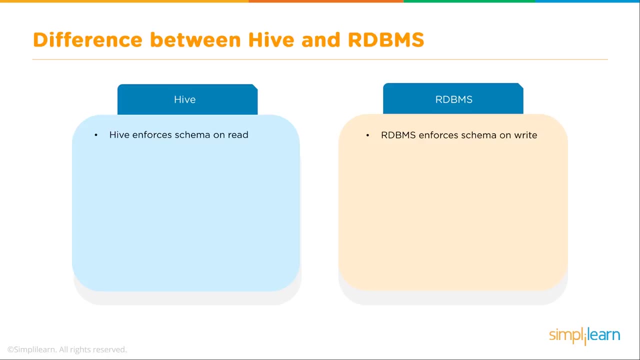 We're looking at ten computers, Fifteen, A hundred, Where this data is spread across all those different Hadoop nodes. Difference between Hive and RDBMS. Remember, RDBMS stands for the Relational Database Management System. Let's take a look at the difference between Hive and the RDBMS. 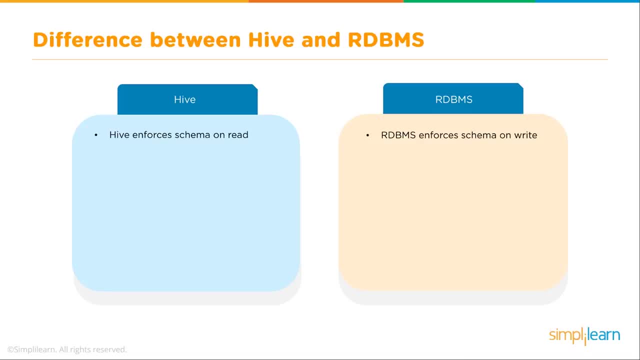 With Hive. Hive enforces schema on read And it's very important that whatever's coming in, that's when Hive's looking at it and making sure that it fits the model. The RDBMS enforces a schema when it actually writes the data into the database. 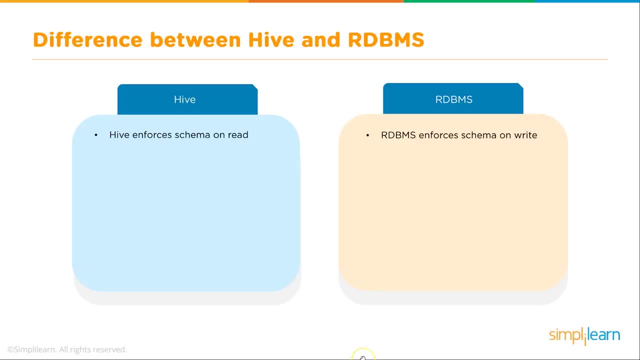 So it's read the data and then, once it starts to write it, that's where it's going to give you the error or tell you something's incorrect about your scheme. Hive data size is in petabytes. That is hard to imagine, You know, when we're looking at your personal computer on your desk, maybe you have ten terabytes if it's a high-end computer. 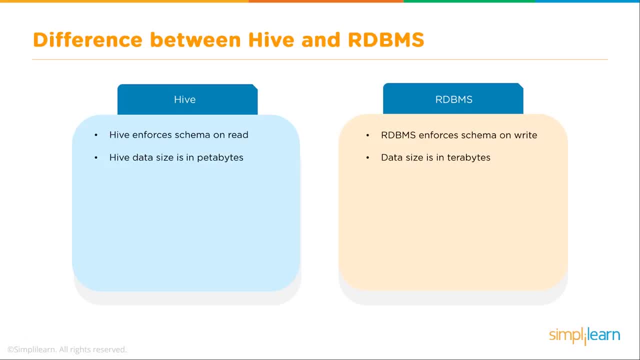 But we're talking petabytes, So that's a lot. So that's hundreds of computers grouped together With RDBMS. data size is in terabytes. Very rarely do you see an RDBMS system that's spread over more than five computers. 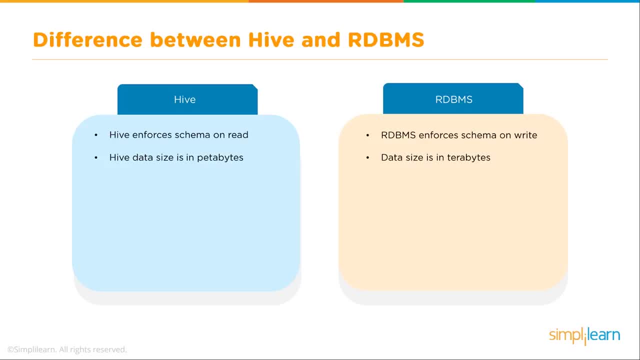 And there's a lot of reasons for that. With the RDBMS, it actually has a high-end amount of writes to the hard drive. There's a lot more going on there. You're writing and pulling stuff. So you really don't want to get too big with an RDBMS or you're going to run into a lot of problems. 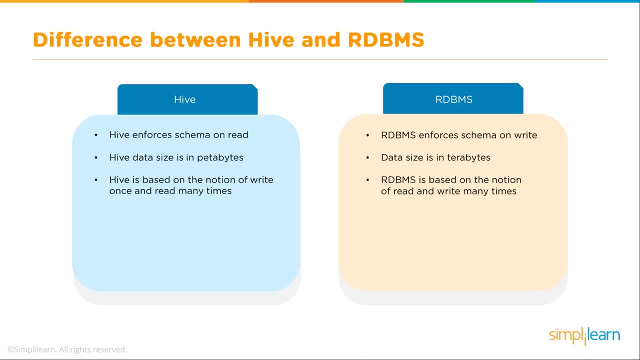 With Hive, you can take it as big as you want. It's based on the notion of write once and read many times. This is so important. They call it WRM, which is write W once O read R many times M. 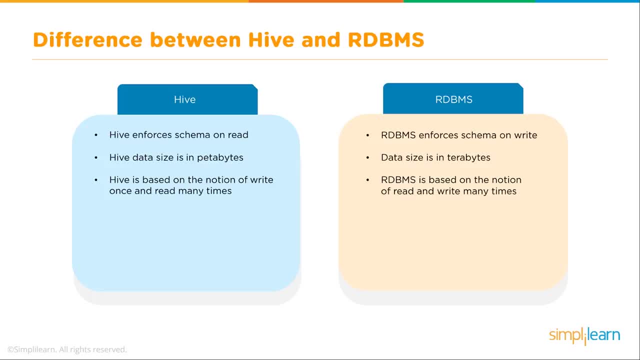 They refer to it as WRM And that's true of a lot of your Hadoop setup. It's altered a little bit But in general, we're looking at archiving data that you want to do data analysis on. We're looking at pulling all that stuff off your RDBMS from years and years and years of business or whatever your company does, or scientific research. 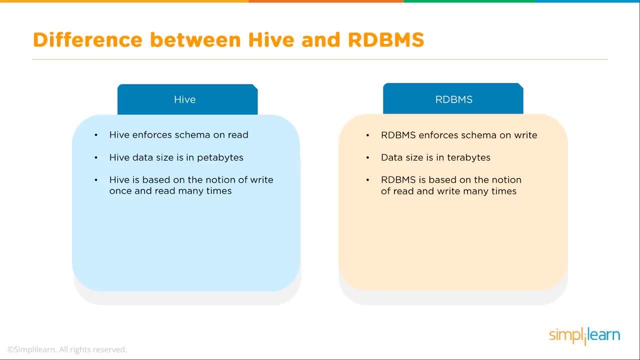 And putting that into a huge database So that you can now do queries on it and get that information out of it. With the RDBMS, it's based on the notion of read and write many times, So you're continually updating this database. 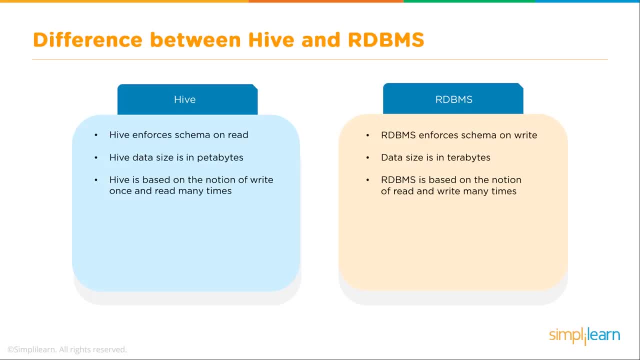 You're continually bringing up new stuff, New sales, The account changes because they have a different licensing. now, Whatever software you're selling All that kind of stuff where the data is continually fluctuating. And then Hive resembles a traditional database by supporting SQL, but it is not a database. 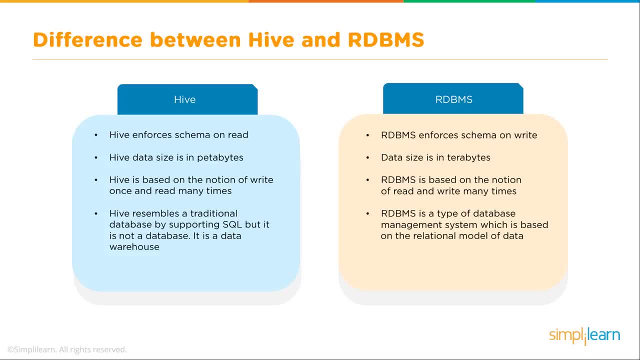 It is a data warehouse. This is very important and it goes with all the other stuff we've talked about, That we're not looking at a database but a data warehouse to store the data and still have fast and easy access to it for doing queries. 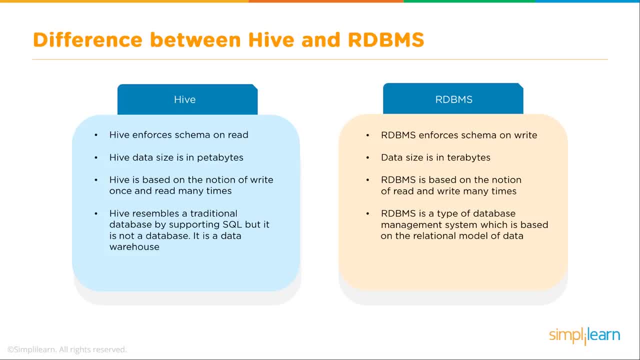 You can think of Twitter and Facebook. They have so many posts that are archived back historically. Those posts aren't going to change. They made the post, They're posted, They're there and they're in their database, But they have to store it in a warehouse in case they want to pull it back up. 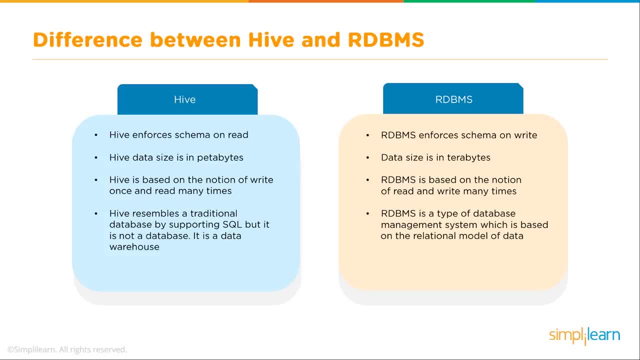 With the RDBMS. it's a type of database management. It's a database management system which is based on the relational model of data And then, with Hive, easily scalable at a low cost- Again we're talking- maybe $1,000 per terabyte. 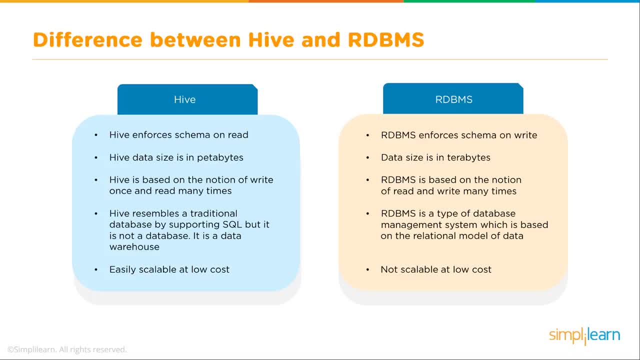 The RDBMS is not scalable at a low cost. When you first start on the lower end, you're talking about $10,000 per terabyte of data, including all the backup on the models and all the added necessities to support it. As you scale it up, you have to scale those computers and hardware up. 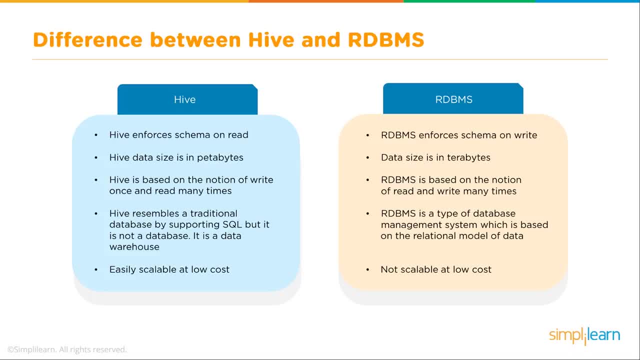 So you might start off with a basic server and then you upgrade to a Sun computer to run it And you spend, you know, tens of thousands of dollars for that hardware upgrade. With Hive, you just put another computer into your Hadoop file system. 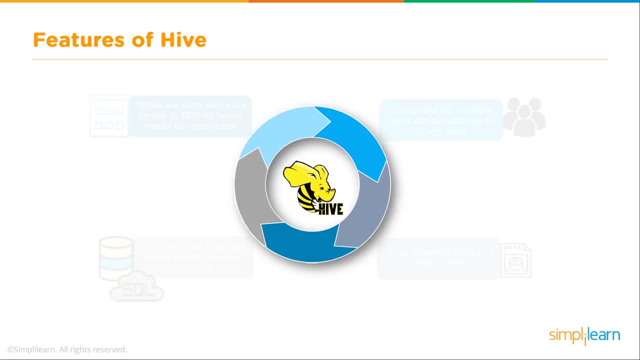 So let's look at some of the features of Hive. When we're looking at the features of Hive, we're talking about the use of SQL-like language called HiveQL. A lot of times you'll see that as HQL, which is easier than long codes. 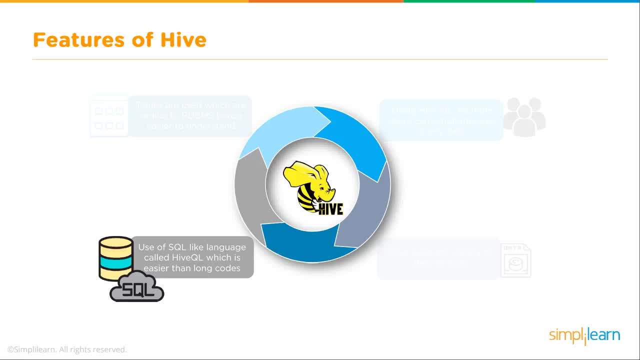 This is nice if you're working with your shareholders. You come to them and you say you can do a basic SQL query on here and pull up the information you need. This way you don't have to have your programmers jump in every time they want to look up something in the database. 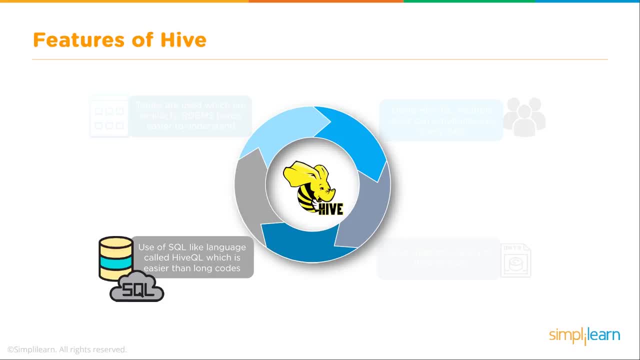 They actually now can easily do that if they're not skilled in programming and script writing. Tables are used which are similar to the RDBMS, hence easier to understand, And one of the things I like about this is when I'm bringing tables in from a MySQL server or SQL server. 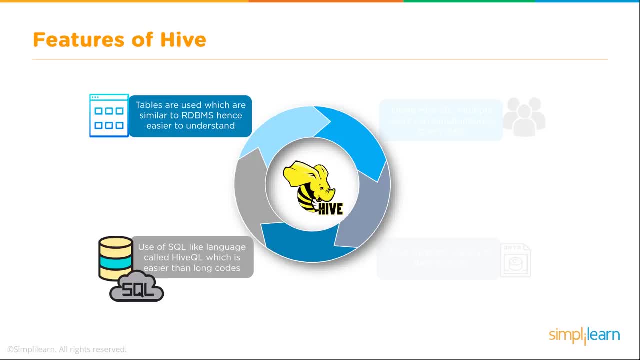 there's almost a direct reflection between the two. So when you're looking at one, which is the data which is continually changing, and then you're going into the archive database, it's not this huge jump where you have to learn a whole new language. 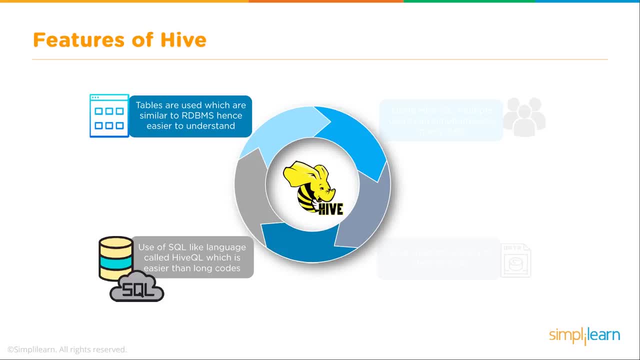 You mirror that same schema into the HDFS, into the Hive, making it very easy to go between the two, And then, using HiveQL, multiple users can simultaneously query data. So again you have multiple clients in there and they send in their query. 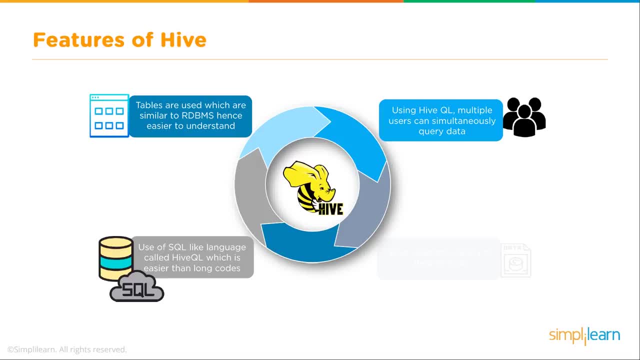 That's also true with the RDBMS, which kind of queues them up. because it's running so fast, you don't notice the lag time. Well, you get that also with the HQL. As you add more computers in the query can go very quickly depending on how many computers. 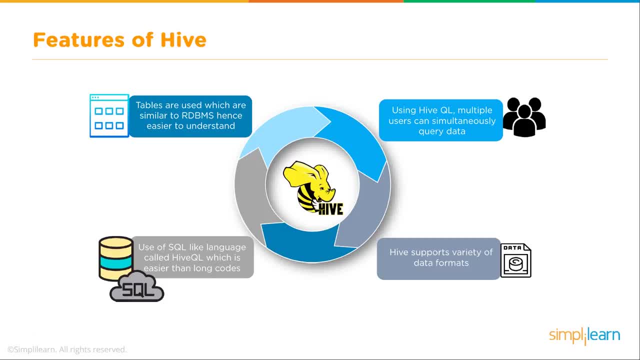 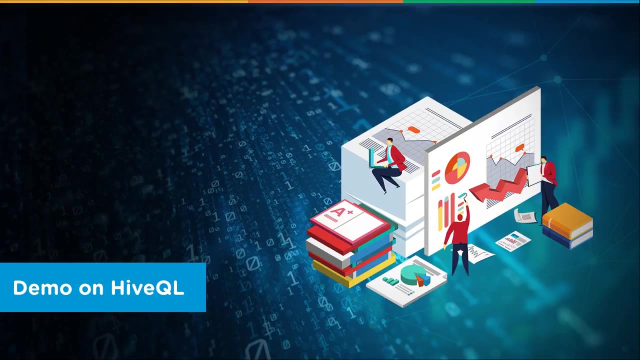 and how much resources each machine has to pull the information. And Hive supports a variety of data types. So with Hive it's designed to be on the Hadoop system, which you can put almost anything into the Hadoop file system. So with all that, let's take a look at a demo on HiveQL or HQL. 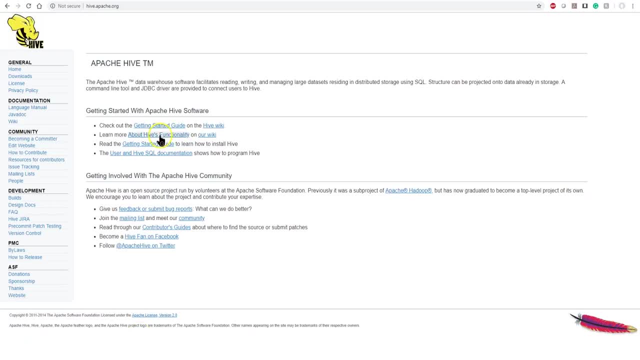 Before I dive into the hands-on demo, let's take a look at the website hiveapacheorg. That's the main website, since Apache. It's an Apache open source software. This is the main software or the main site for the build. 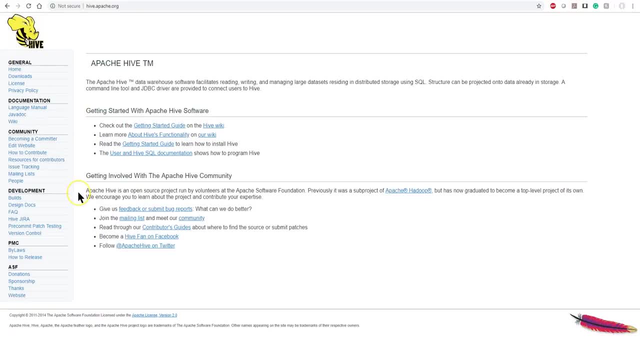 And if you go in here you'll see that they're slowly migrating Hive into Beehive. And so if you see Beehive versus Hive, note that Beehive is the new releases coming out. That's all it is. It reflects a lot of the same functionality of Hive. 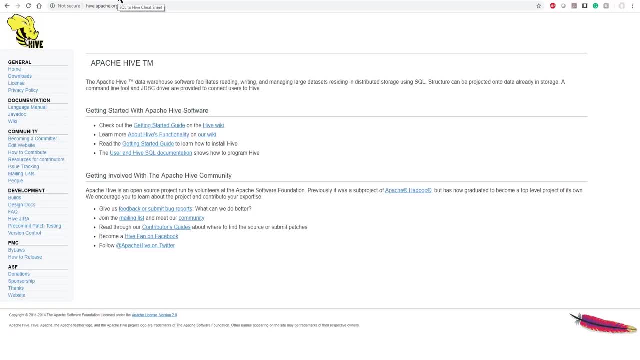 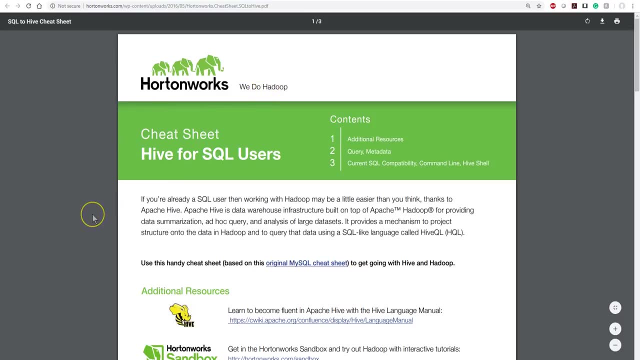 It's the same thing. And then we like to pull up some kind of documentation on commands, And for this I'm actually going to go to Hortonworks Hive cheat sheet, And that's because Hortonworks and Cloudera are two of the most common used builds for Hadoop. 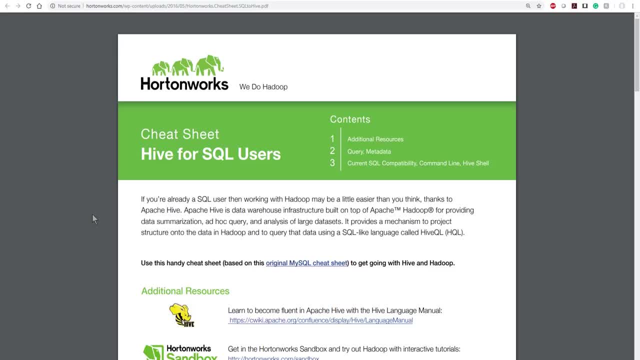 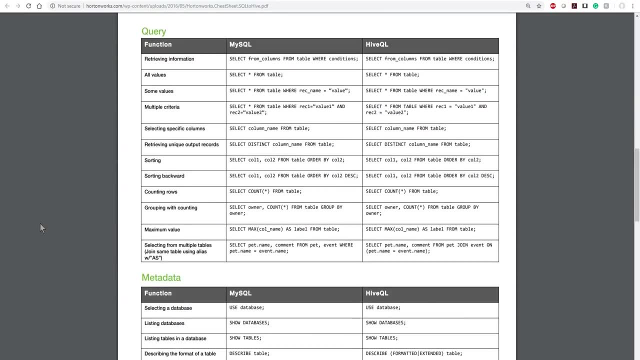 and for which include Hive and all the different tools in there, And so Hortonworks has a pretty good PDF. you can download cheat sheet on there. I believe Cloudera does too, But we'll go ahead and just look at the Horton one, because it's the one that comes up really good. 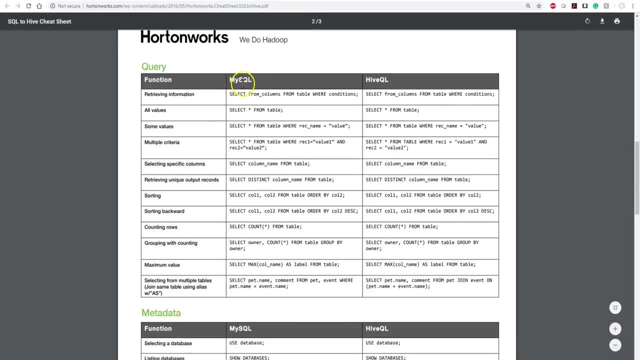 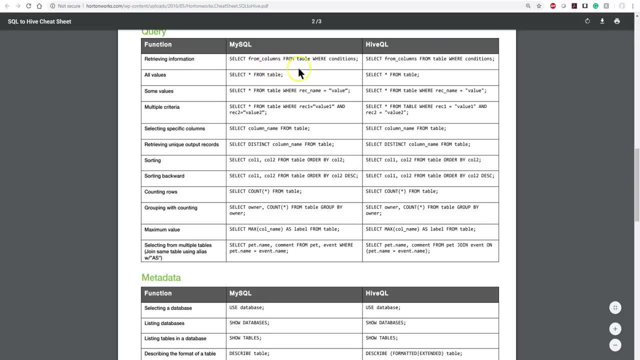 And you can see when we look at the query language it compares MySQL Server to HiveQL. And you can see the basic select. We select from columns, from table where conditions exist. You know most basic command on there And they have different things. you can do with it just like you do with your SQL. 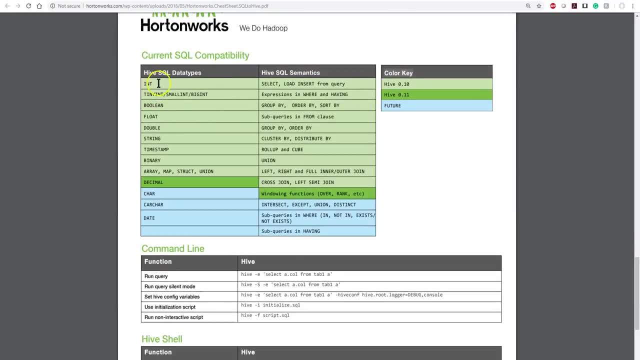 And if you scroll down you'll see data types. So here's your integer, your flow, your binary double string time stamp and all the different data types. you can use Some different semantics, different keys, features, functions for running a Hive query. 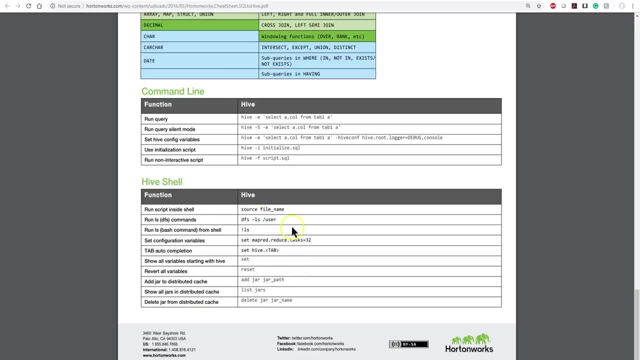 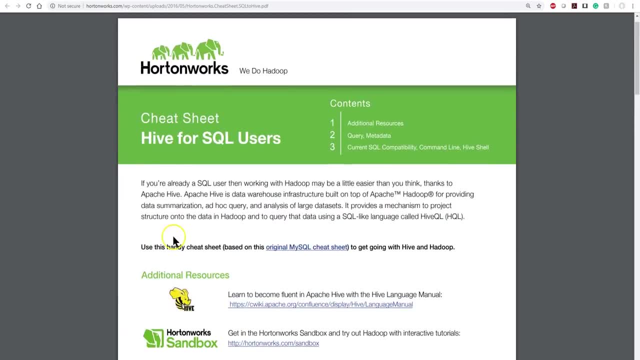 Command line set up And of course the Hive shell set up in here. So you can see right here, if we loop through it, it has a lot of your basic stuff in it. So we're basically looking at SQL across a Horton database. 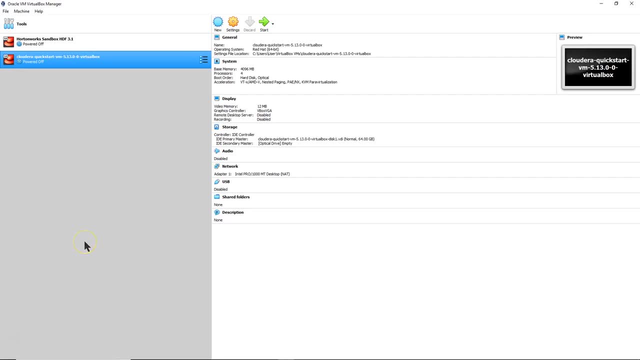 We're going to go ahead and run our Hadoop cluster Hive demo And I'm going to go ahead and use the Cloudera quick start And this is in the virtual box. So again, we have an Oracle virtual box which is open source. 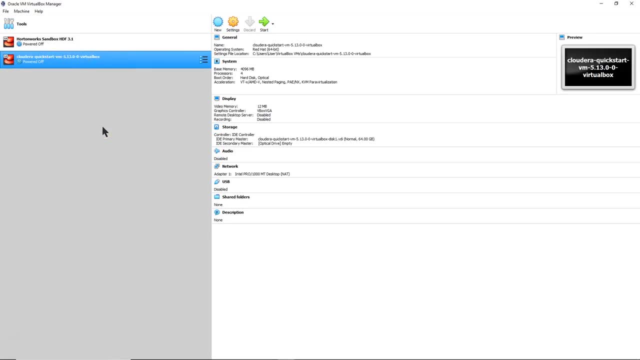 And then we have our Cloudera quick start, which is the Hadoop set up on a CPU, Hadoop set up on a single node. Now, obviously, Hadoop and Hive are designed to run across a cluster of computers, So when we talk about a single node it's for education, testing, that kind of thing. 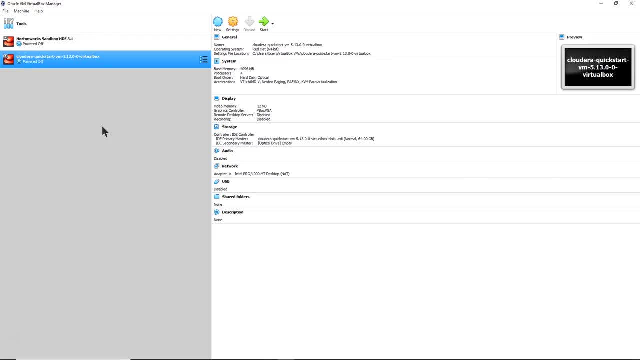 And if you have a chance, you can always go back and look at our demo we had on setting up a Hadoop system in a single cluster. Just set a note down below in the YouTube video And our team will get in contact with you and send you that link if you don't already have it. 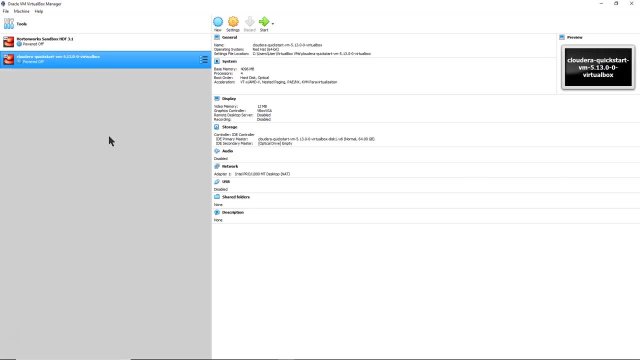 Or you can contact us at the wwwsimplylearncom. Here. it's always important to note that you do need on your computer- if you're running on Windows- because I'm on a Windows machine- you're going to need probably about 12 gigabytes to actually run this. 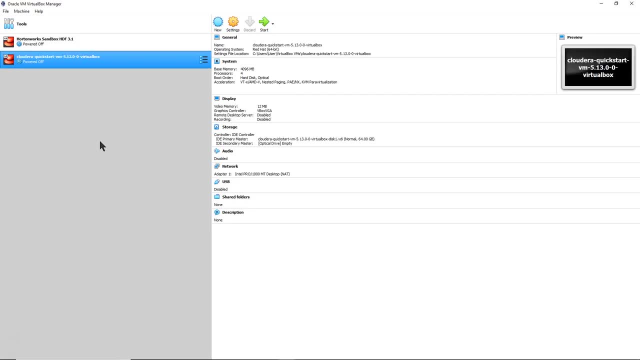 It used to be, you could buy with a lot less, but as things have evolved they take up more and more resources And you need the professional version If you have the home version. I was able to get that to run, but boy did it take a lot of extra work to get the home version to. let me use the virtual set up on there. 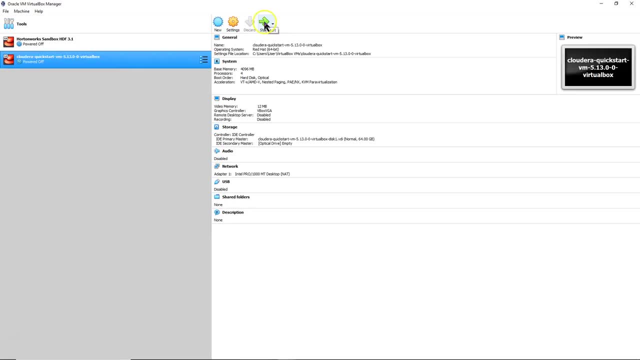 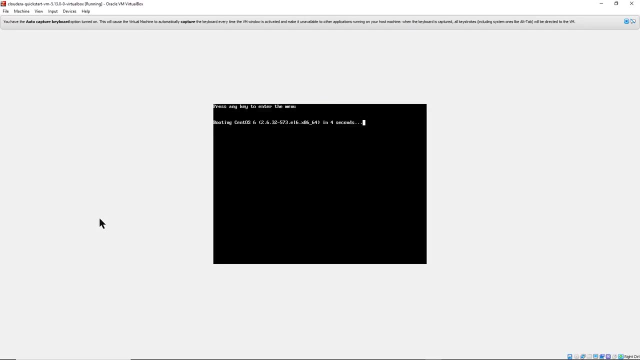 And we'll simply click on the Cloudera quick start And I'm going to go ahead and just start that up. And this is starting up our Linux. So we have our Windows 10, which is the computer I'm on, And then I have the VirtualBox, which is going to have a Linux operating system in it. 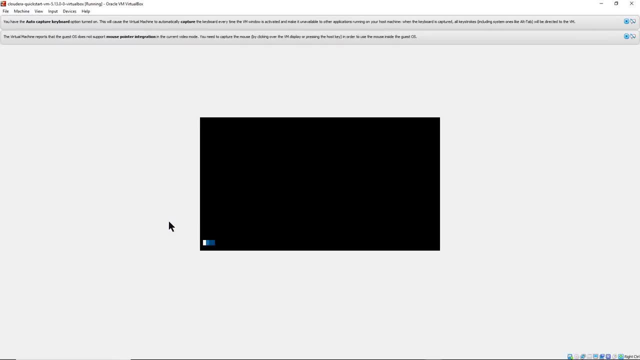 And we'll skip ahead, so you don't have to watch the whole install. Something interesting to know about the Cloudera is that it's running on Linux CentOS And, for whatever reason, I've always had to click on it and hit the escape button for it to spin up. 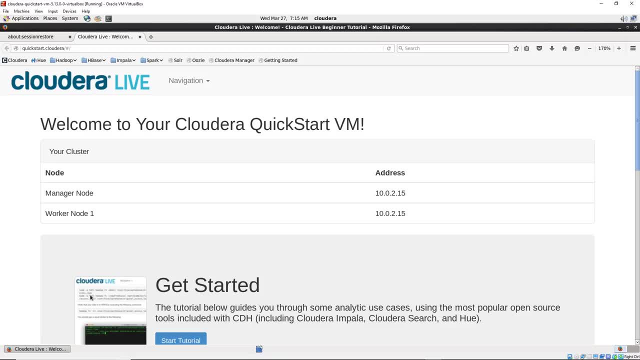 And then you'll see the DOS come in here. Now that our Cloudera is spun up on our virtual machine with the Linux on, we can see here it uses the Thunderbird browser on here by default and automatically opens up a number of different tabs for us. 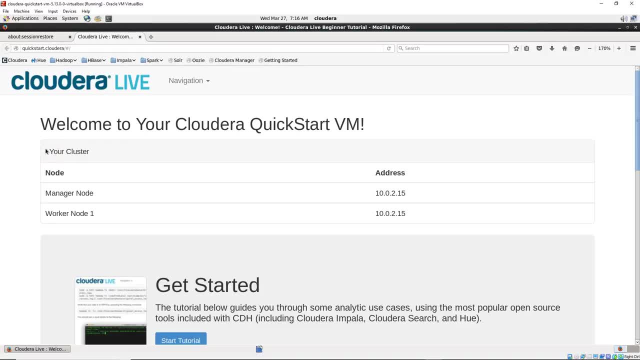 And a quick note, because I mentioned the restrictions on getting set up on your own computer. If you have a home edition computer and you're worried about setting it up on there, you can also go in there and spin up a one month free service on Amazon Web Service to play with this. 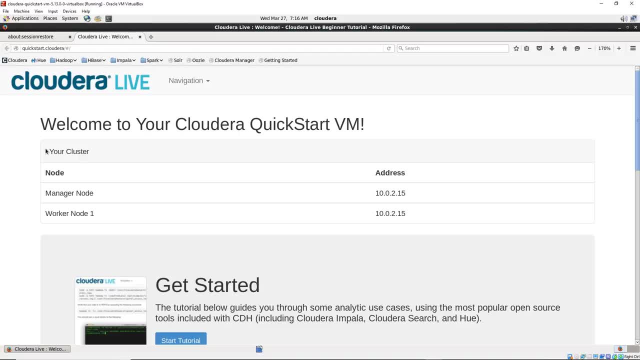 So there's other options. You're not stuck with just doing it on the quick start menu. You can spin this up in many other ways. Now, the first thing we want to note is that we've come in here into Cloudera and I'm going to access this in two ways. 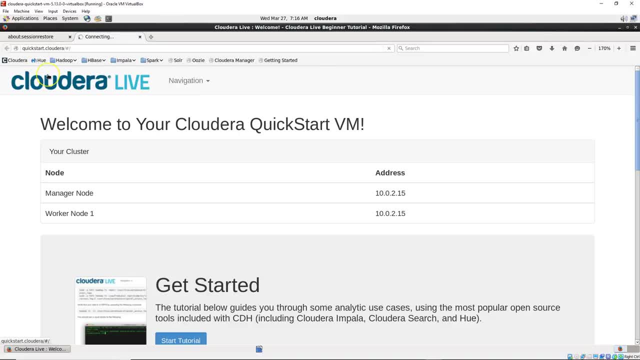 The first one is we're going to use Hue And I'm going to open up Hue and it'll take it a moment to load from the setup on here And Hue is nice If I go in and use Hue as an editor into Hive or into the Hadoop setup. 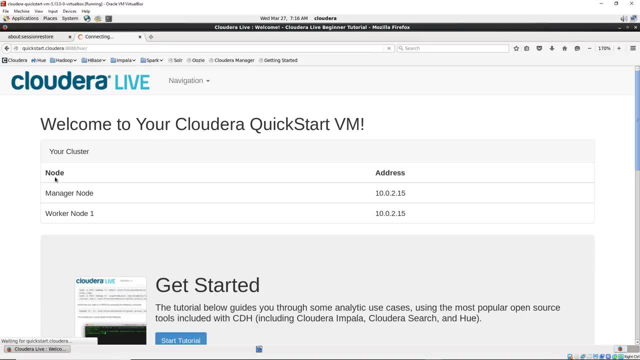 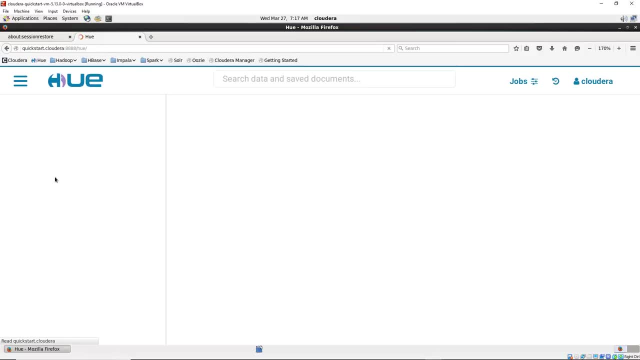 usually I'm doing it from an admin side, because it has a lot more information, a lot of visuals, Less to do with actually diving in there and just executing code. And you can also write this code into files and scripts and there's other ways you can upload it into Hive. 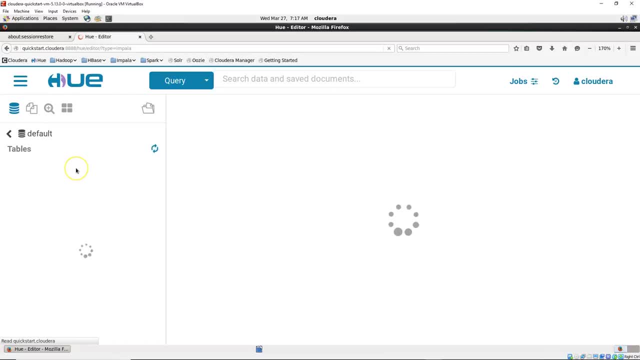 But today we're going to look at the command lines and we'll upload it into Hue and then we'll go into and actually do our work in a terminal window under the Hive shell. Now in the Hue browser window, if you go under query and click on the pull down menu, 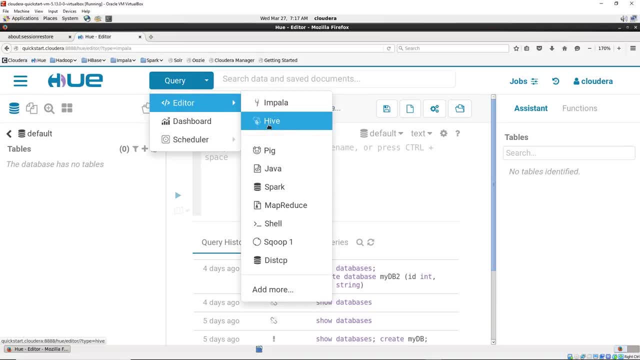 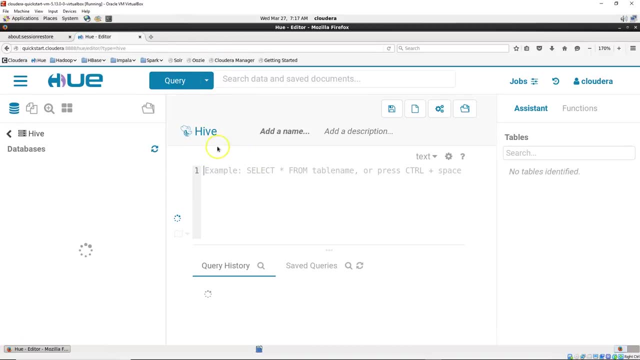 and then you go under editor and you'll see Hive. There we go. There's our Hive setup. I go and click on Hive and this will open it up. We've got our query down here and now it has a nice little B that shows our Hive going. 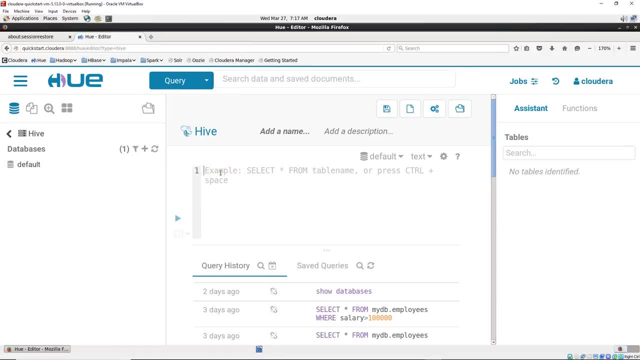 and we can go something very simple down here, like show databases, and we follow it with a semicolon, And that's the standard in Hive is you always add our punctuation at the end there And I'll go ahead and run this and the query will show up underneath. 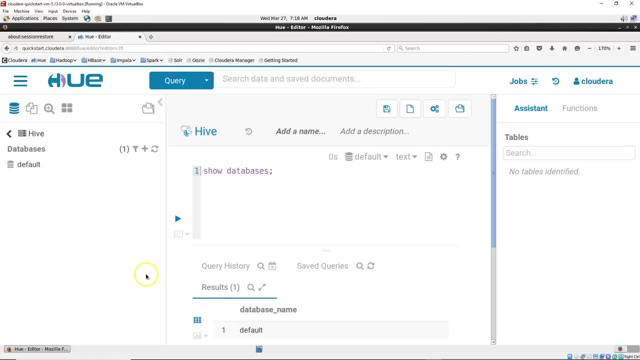 And you'll see down here, since this is a new quick start I just put on here. you'll see. it has the default down here for the databases. That's the database name. I haven't actually created any databases on here. And then there's a lot of other like assistant function. tables your databases up here. 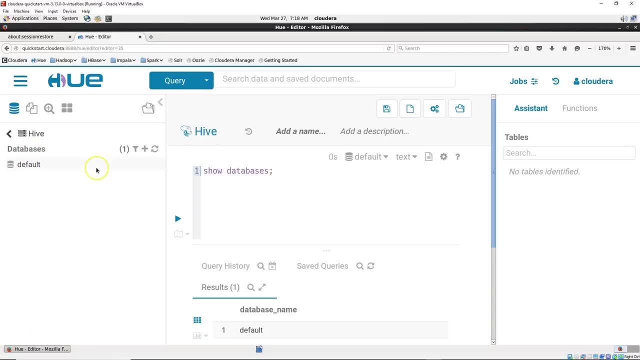 There's all kinds of things you can look at through Hue as far as a bigger picture. The downside of this is it always seems to lag For me. whenever I'm doing this, I always seem to run slow. So if you're in Cloudera you can open up a terminal window. 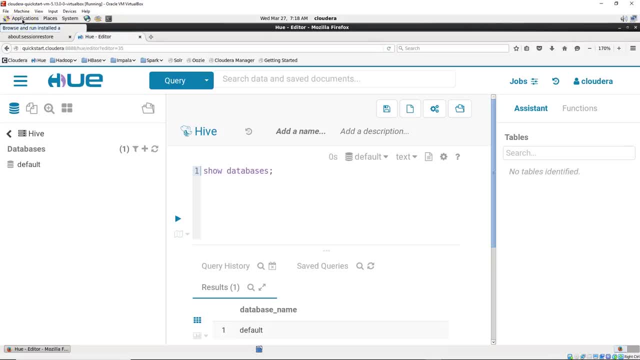 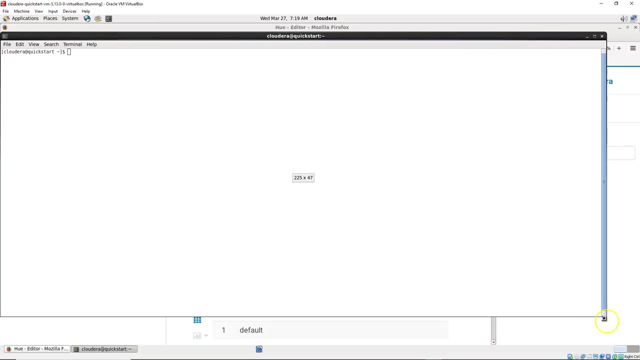 They actually have an icon at the top. You can also go under applications and under applications, system tools and terminal. Either one will work. It's just a regular terminal window And this terminal window is now running underneath our Linux. So this is a Linux terminal window on our virtual machine, which is resting on our regular Windows 10 machine. 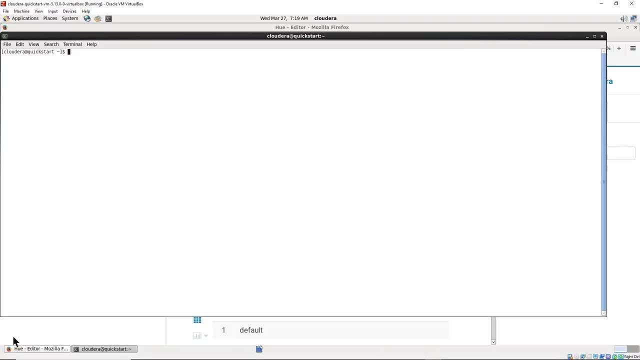 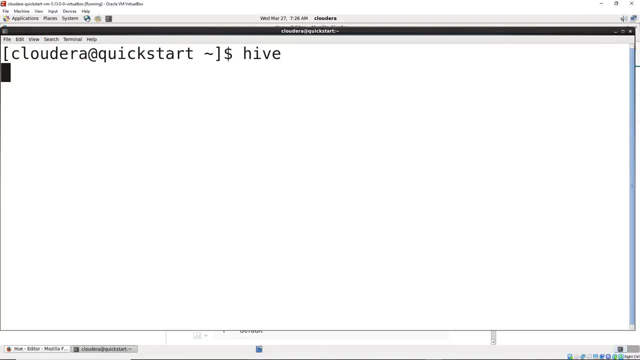 And we'll go ahead and zoom this in so you can see the text better on your own video. And I simply just clicked on view and zoom in And then all we have to do is type in Hive And this will open up the shell on here. 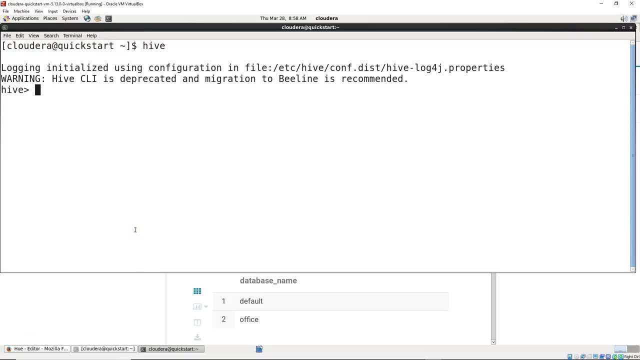 And it takes it just a moment to load. When starting up Hive, I also want to note that, depending on your rights on the computer you're on and your action, you might have to do sudo hive and put in your password and username. Most computers are usually set up with the Hive login. 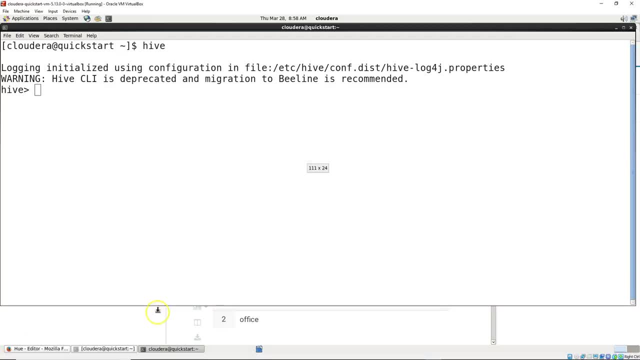 Again, it just depends on how you're accessing the Linux system and the Hive shell. Once we're in here, we can go ahead and do a simple HQL command- Show databases, And if we do that we'll see here that we don't have any databases. 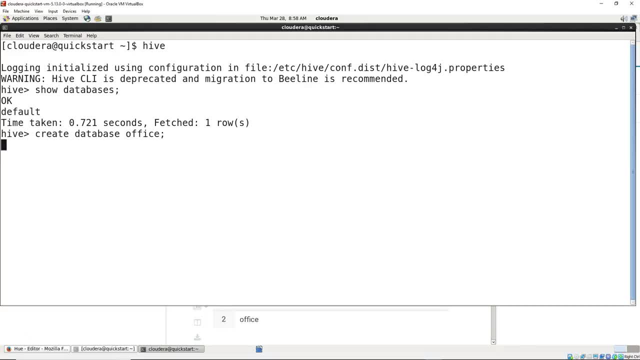 So we can go ahead and create a database And we'll just call it Office for this moment. Now, if I do show, we'll just do the up arrow. Up arrow is a hotkey that works in both Linux and in Hive, So I can go back and page through all the commands I've typed in. 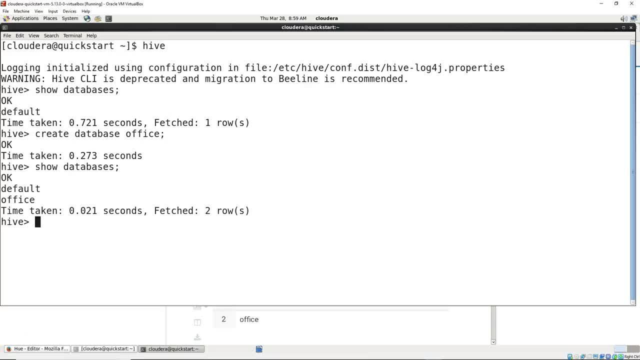 And we can see now that I have my. there's, of course, the default database And then there's the Office database. So now we've created a database. It's pretty quick and easy And we can go ahead and drop the database. 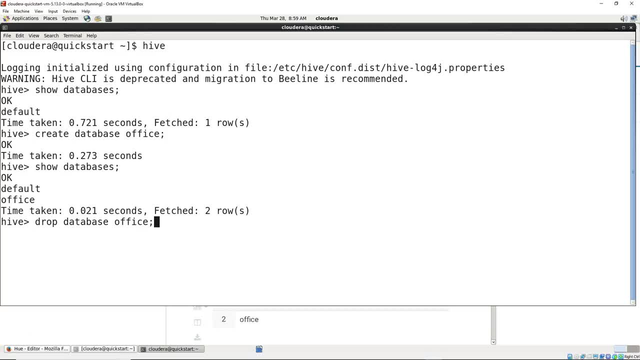 We can do drop database Office. Now this will work on this database because it's empty. If your database was not empty, you would have to do cascade And that drops all the tables in the database and the databases. Now, if we do show database, 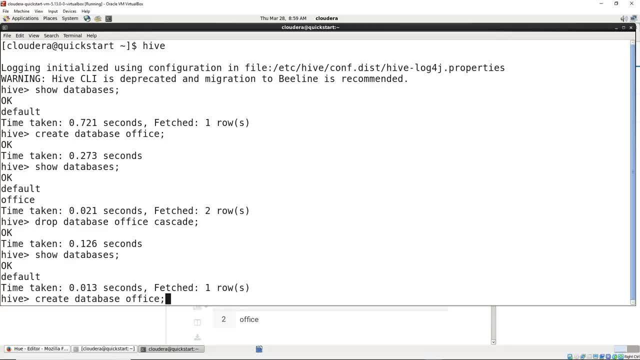 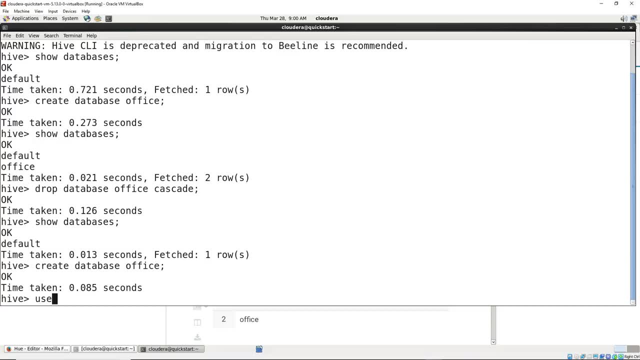 And we'll go ahead and recreate our database Because we're going to use the Office database for the rest of this hands on demo. A really handy command, now set with the SQL or HQL, is to use Office, And what that does is that sets Office as the default database. 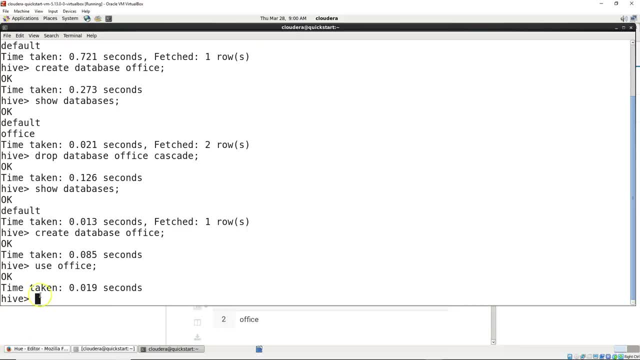 So, instead of having to reference the database every time we work with a table, It now automatically assumes that's the database being used for whatever tables we're working on. The difference is you put the database name period table And I'll show you in just a minute what that looks like and how that's different. 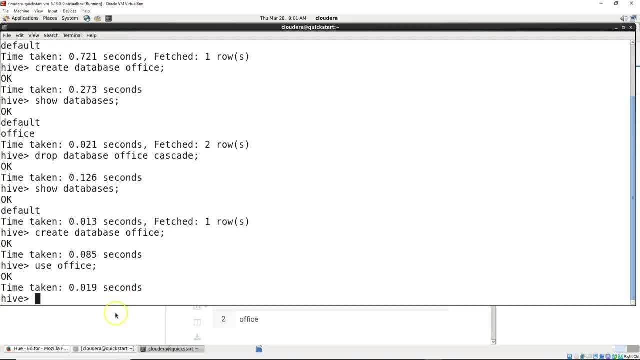 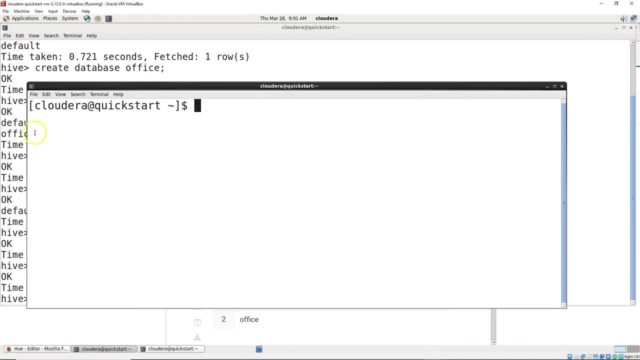 If we're going to have a table and a database, we should probably load some data into it. So let me go ahead and switch gears here And open up a terminal window. You can just open another terminal window and it'll open up right on top of the one that you have Hive Shell running in. 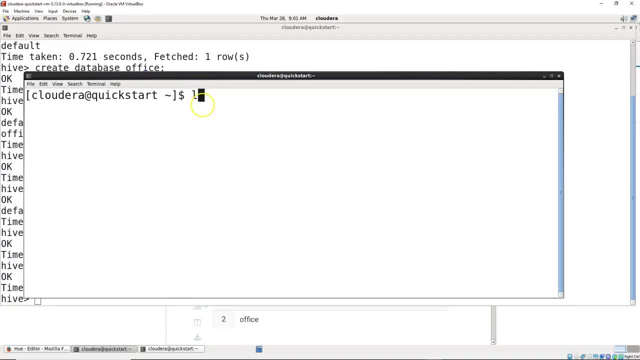 And when we're in this terminal window. First we're going to go ahead and just do a list, Which is, of course, a Linux command. You can see all the files I have in here. This is the default load. We can change directory to documents. 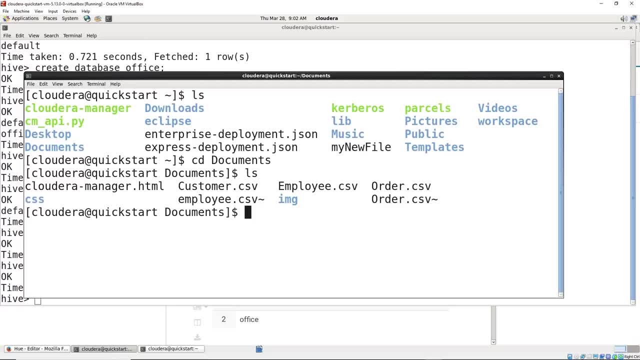 We can list in documents And we're actually going to be looking at employeecsv. A Linux command is the cat. You can use this actually to combine documents. There's all kinds of things that cat does. But if we want to just display the contents of our employeecsv file, 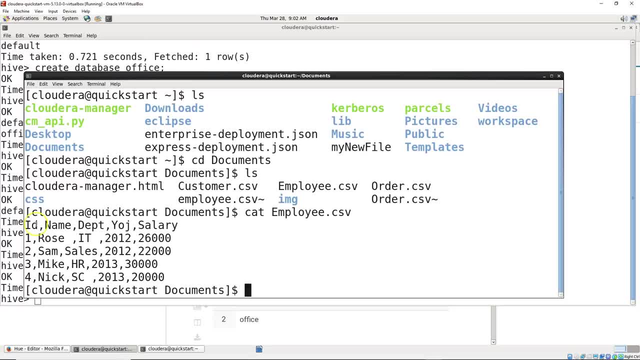 We can simply do cat employee csv, And when we're looking at this, we want to know a couple things. One: there's a line at the top, Okay, So the very first thing we notice Is that we have a header line. 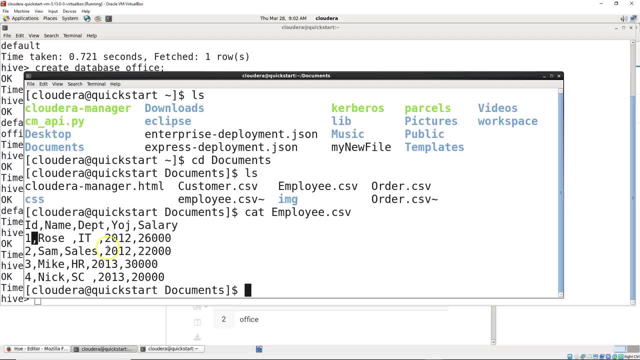 The next thing we notice is that the data is comma separated And in this particular case you'll see a space here. Generally with these you've got to be real careful with spaces. There's all kinds of things you've got to watch out for. 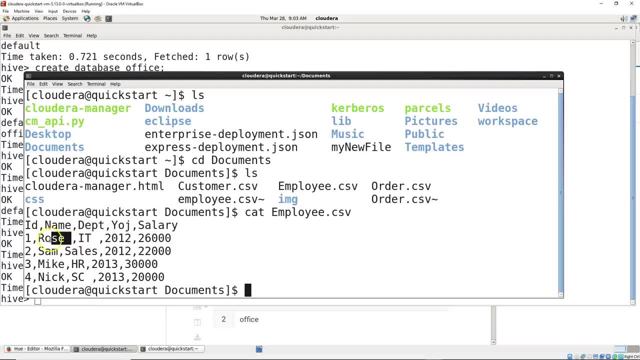 Because it can cause issues. These spaces won't Because these are all strings that the space is connected to. If this was a space next to the integer, You would get a null value that comes into the database Without doing something extra in there. 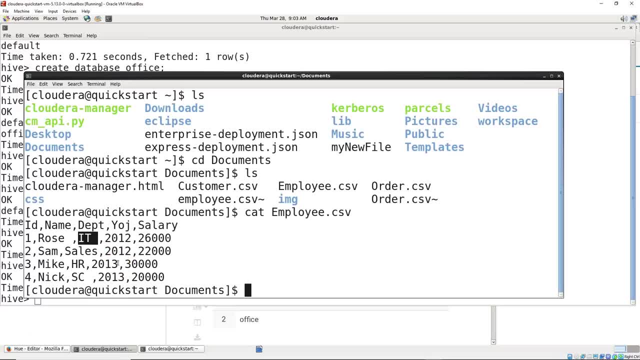 Now with most of Hadoop, that's important to know. You're writing the data once, Reading it many times, And that's true of almost all your Hadoop things coming in. So you really want to process the data before it gets into the database. 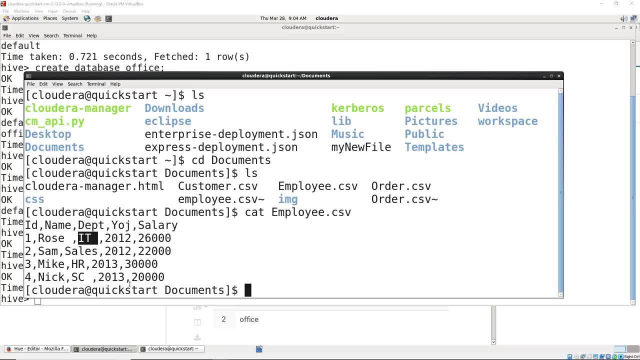 And for those of you who have studied data transformation, That's the etl, Where you extract transfer form And then load the data. So you really want to extract and transform before putting it into the hive. Then you load it into the hive with the transformed data. 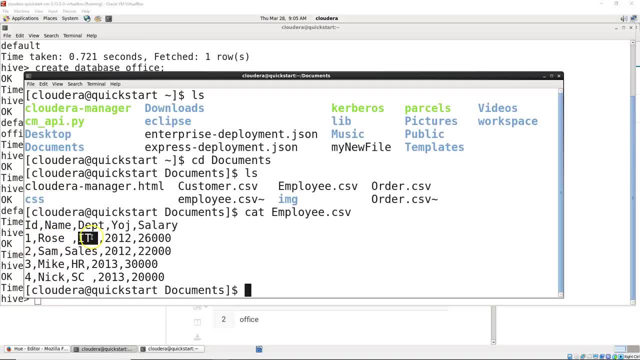 And, of course, we also want to note the schema. We have an integer String, Integer, Integer, So we kept it pretty simple in here As far as the way the data is set up- The last thing that you're going to want to look up- 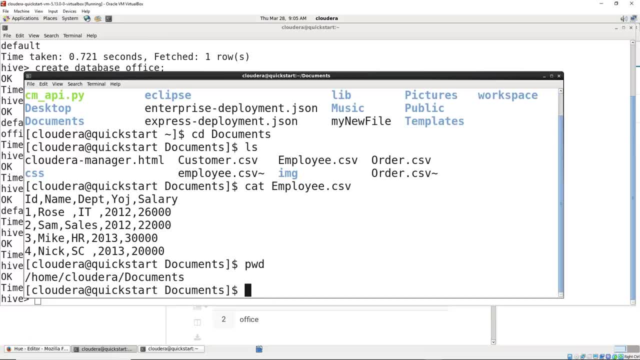 Is the source. Since we're doing local uploads, We want to know what the path is. We have the whole path. In this case it's home Slash, Cloudera, Slash Documents, And these are just text documents We're working with right now. 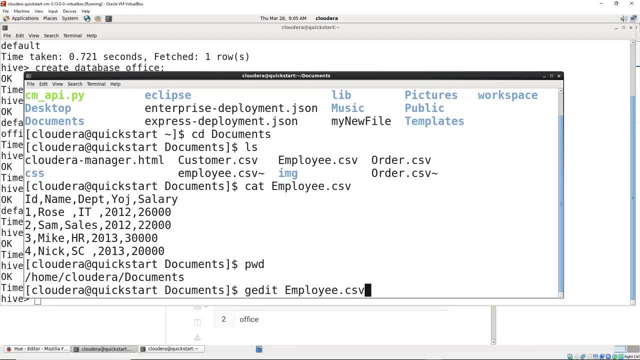 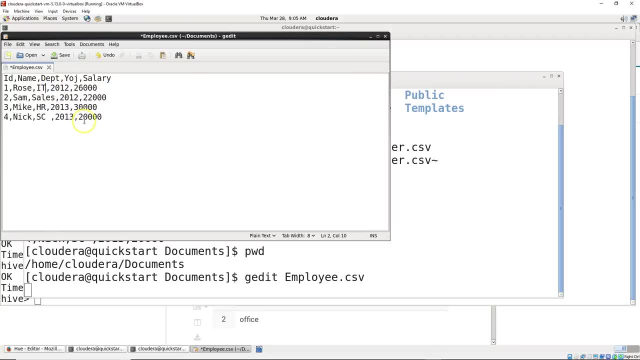 We're not doing anything fancy. So we can do a simple get edit Employee CSV And you'll see it comes up here. It's just a text document, So I can easily remove these edits. There we go, And then we go ahead and just save it. 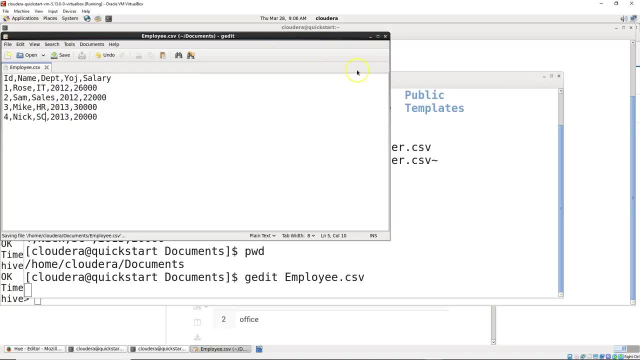 And so now it has the new setup in there. We've edited it. The gedit is usually one of the default that loads into Linux, So any text editor will do Back to the hive shell. So let's go ahead and create a table. 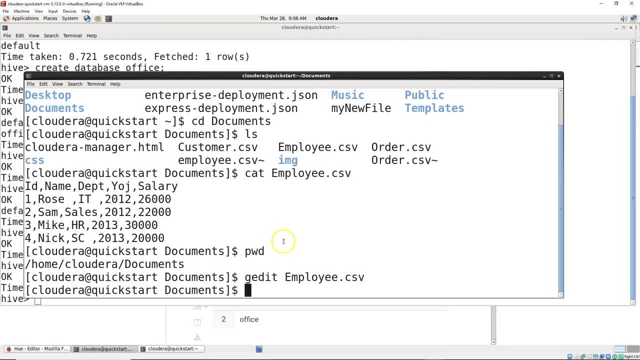 Employee. And what I want you to note here Is I did not put the semicolon on the end here. Semicolon tells it to execute that line. So this is kind of nice. If you're, You can actually just paste it in. 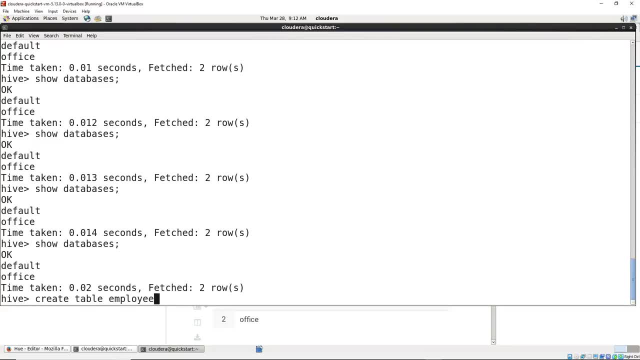 If you have it written on another sheet. And you can see right here Where we have the table And you can see right here Where we have the table. And you can see right here Where we have the table. And you can see right here. 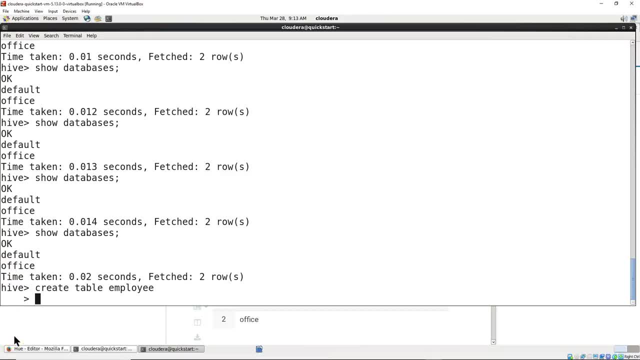 Where I have create table employee And it goes into the next line on there, So I can do all of my commands at once. Now, just so I don't have any typo errors, I went ahead and just pasted the next three lines in. 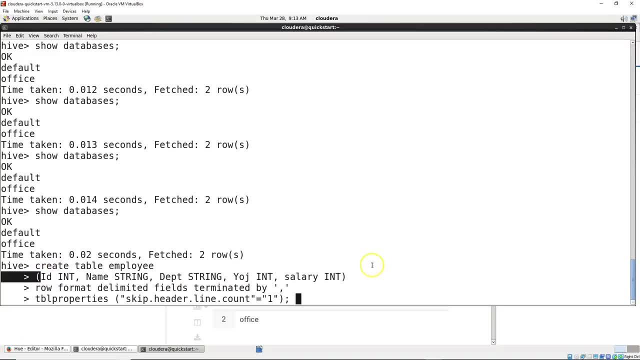 And the next one is our schema. If you remember correctly from the other side, We had the different values in here, Which was id name, department, year of joining And salary, And the id is an integer, Name is a string. 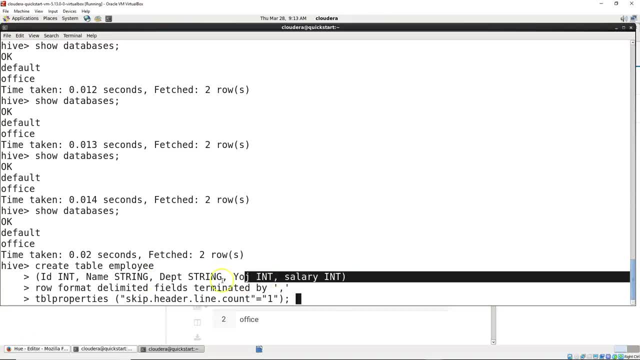 Department is string, Year of joining, Salary is an integer And they're in brackets, So we put close black brackets around them And you could do this all as one line. And then we have row format: delimited fields terminated by comma, And this is important because the default is tabs. So if I do it now, 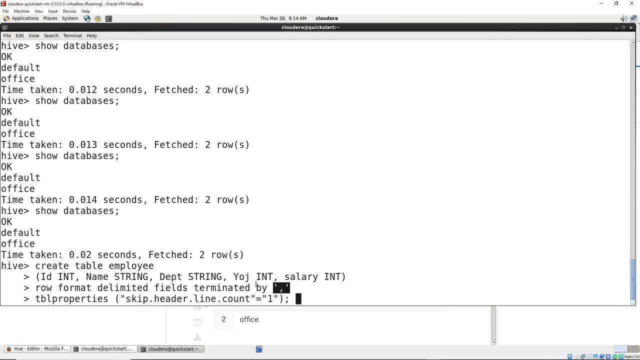 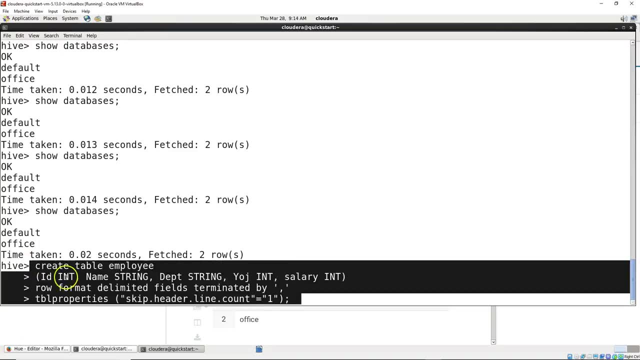 it won't find any terminated fields, So you'll get a bunch of null values loaded into your table. And then finally, our table properties. we want to skip the header line. count equals one. Now this is a lot of work for uploading a single file. It's kind of goofy when you're uploading. 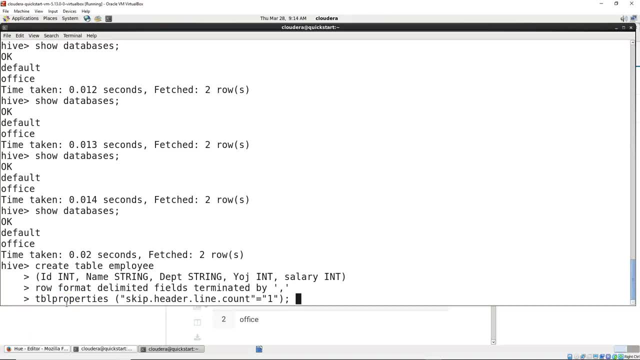 a single file, that you have to put all this in here. But keep in mind Hive and Hadoop is designed for writing many files into the database. You write them all in there and then you can. they're saved. It's an archive, It's a data warehouse, And then you're able to do all your queries on them. 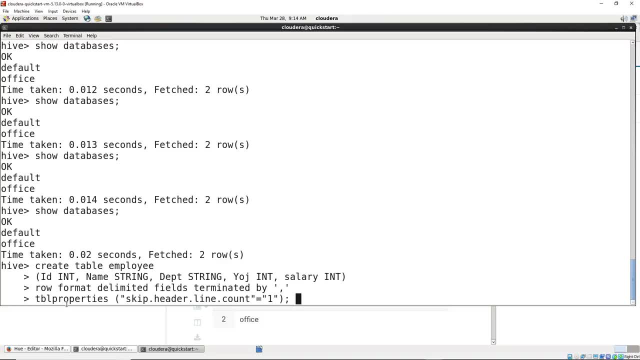 So a lot of times we're not looking at just the one file coming up, We're loading hundreds of files. You have your reports coming off of your main database. All those reports are being loaded. You have your log files, You have, I mean, all this different data is being dumped into Hadoop. 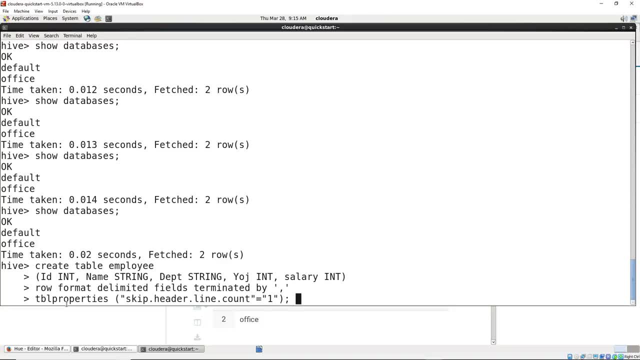 and in the database, And then you have all the files that you're loading into Hadoop. And then you have all the files that you're loading into Hadoop. And then you have all the files that you're loading into Hadoop- In this case Hive on top of Hadoop- And so we need to let it know. hey, how do I handle these files? 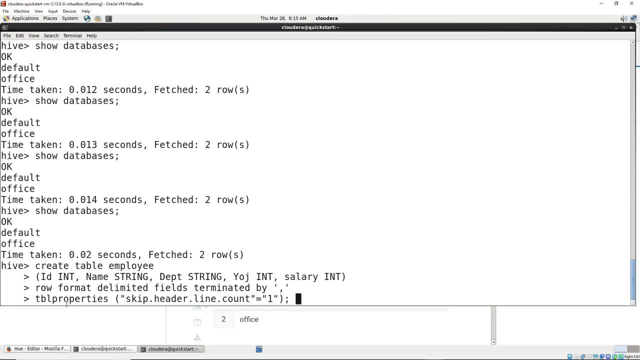 coming in, And then we have the semicolon at the end which lets us know to go ahead and run this line. And so we'll go ahead and run that. And now, if we do a show tables, you can see, there's our 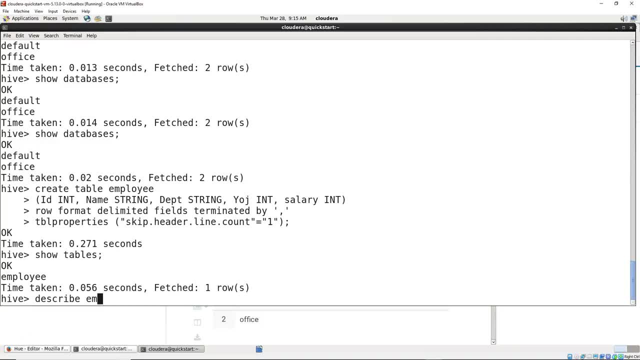 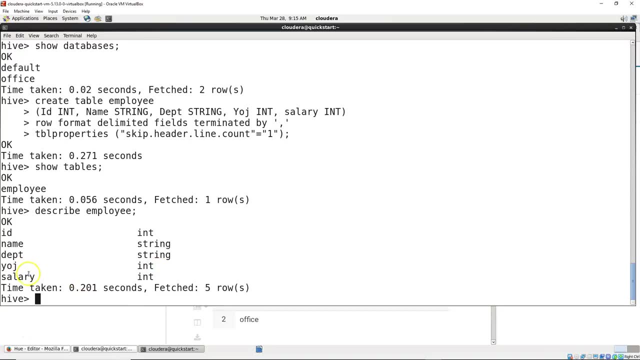 employee on there We can also describe. If we do describe employee, you can see that we have our ID, integer, name, string, department, string, year of joining integer and salary: integer. And then, finally, let's just do a select star from: 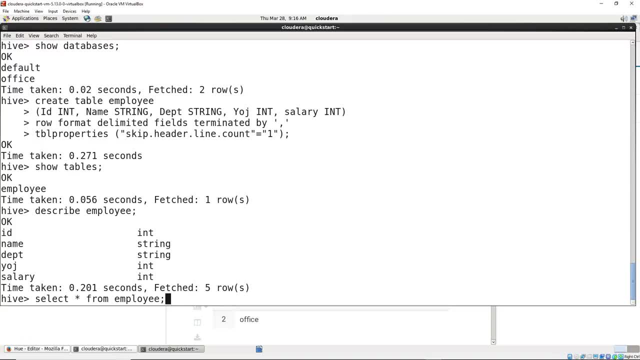 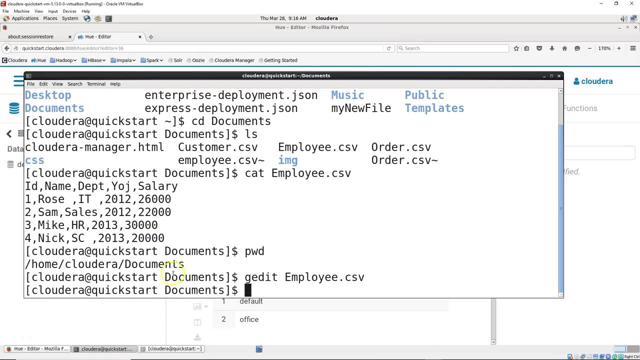 employee, very basic SQL and HQL command selecting data And it's going to come up and we haven't put anything in it. So, as we expect, there's no data in it. So if we flip back to our Linux terminal window, you can see where we did the cat employeecsv And you can 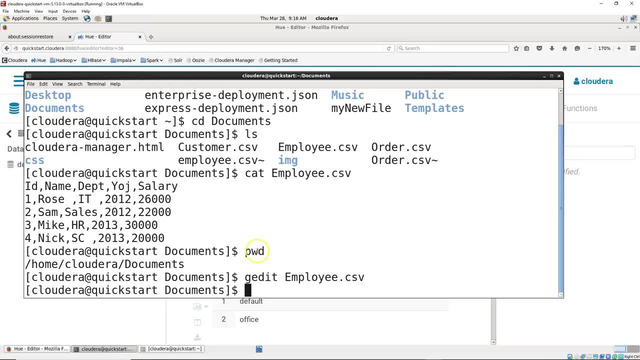 see all the data we expect to come into it And we also did our PWD And right here you see the path. You need that full path. when you are loading data, You know you can do a browse and if I did it right now with just the employeecsv as a name, it will work, But that is. 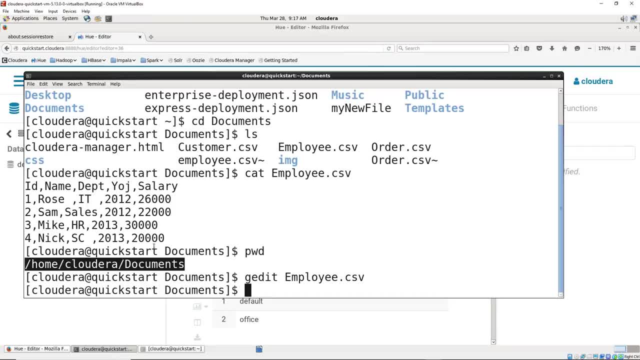 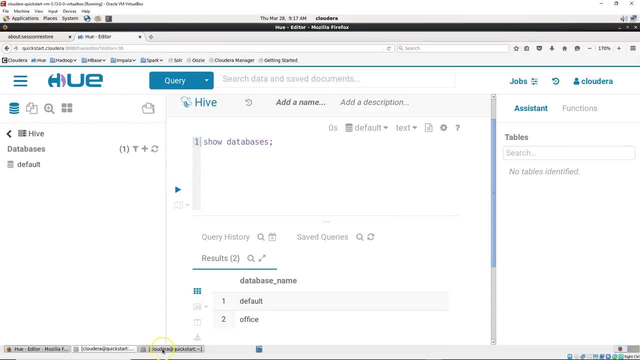 a really bad habit In general when you're loading data, because it's you don't know what else is going on in the computer. you want to do the full path almost in all your data loads, So let's go ahead and flip back over here to our hive shell. we're working in And the command for this is: 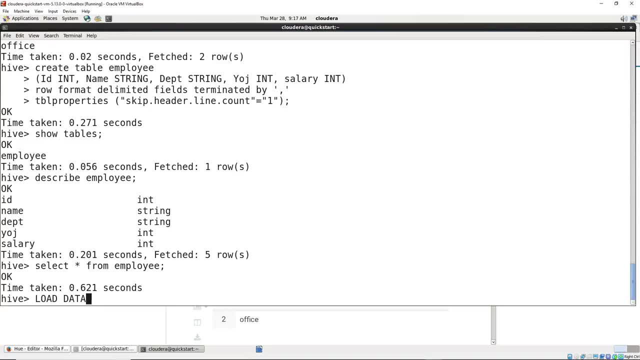 load data. So that says, hey, we're loading data, That's a hive command, HQL, And we want local data. So you got to put down local and path. So now it needs to know where the path is. So we're going to. 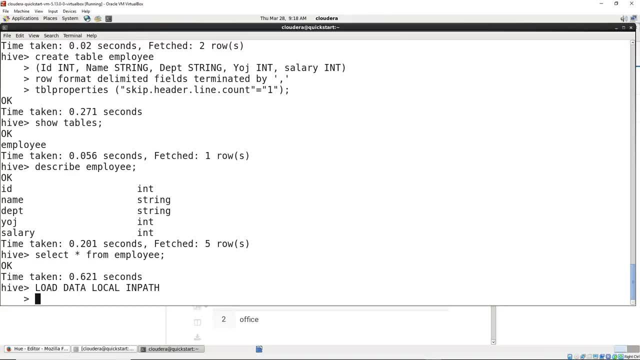 do this Now to make this more legible. I'm just going to go ahead and hit enter And then we'll just paste the full path in there, which I have stored over on the side like a good prepared demo, And 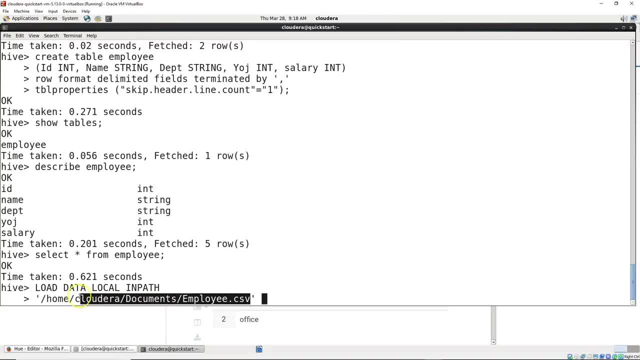 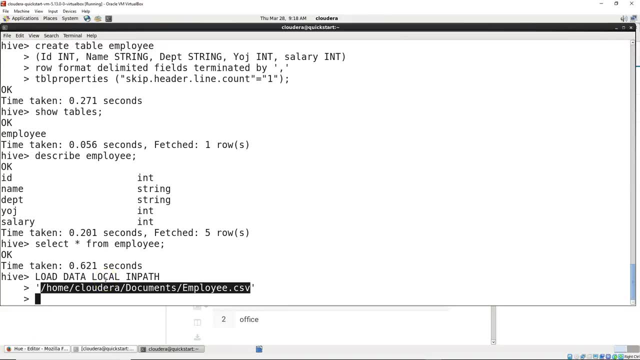 you'll see here we have home Cloudera documents- employeecsv- So it's a whole path for this text document in here And we go ahead and hit enter in there And then we have to let it know where the data is going. So now we have a source and we need a destination And it's going to go into 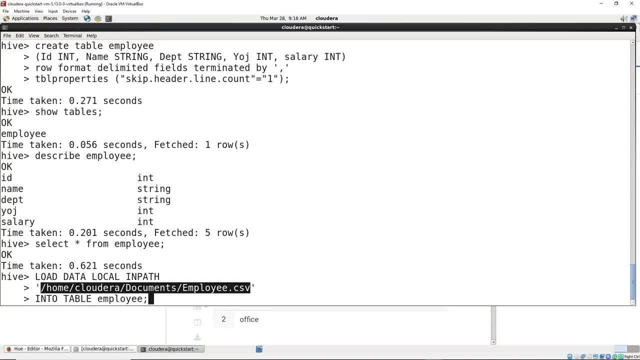 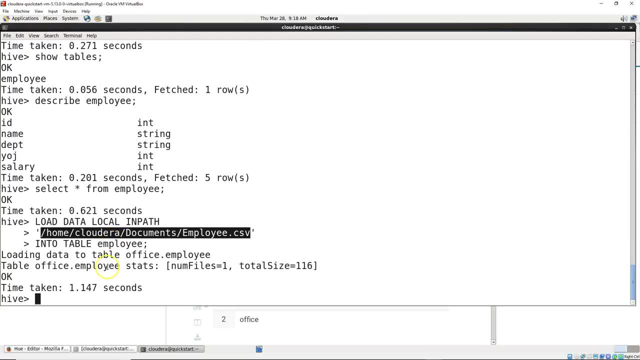 the table and we'll just call it employee. We'll just match the table in there And because I wanted to execute, we put the semicolon on the end. It goes ahead and executes all three lines. Now, if we go back, if you remember, we did the select star from employee just using the up error to page. 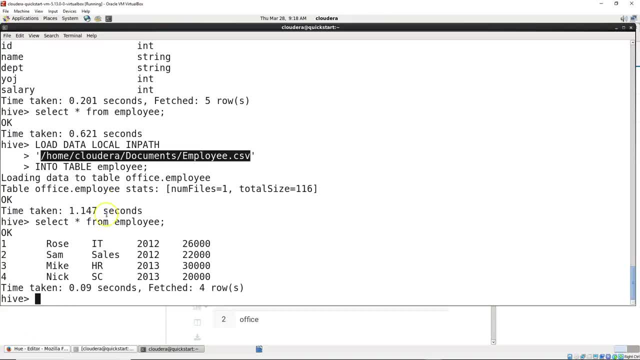 through my different commands I've already typed in. You can see right here we have as we expect. we have Rose, Sam, Mike and Nick And we have all their information showing in our four rows. And then let's go ahead and do select and count. We'll just look at a couple of these different 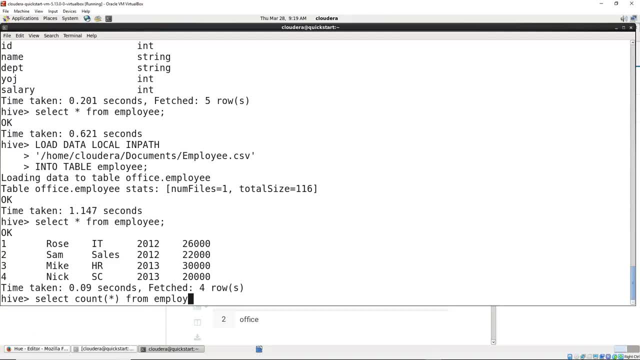 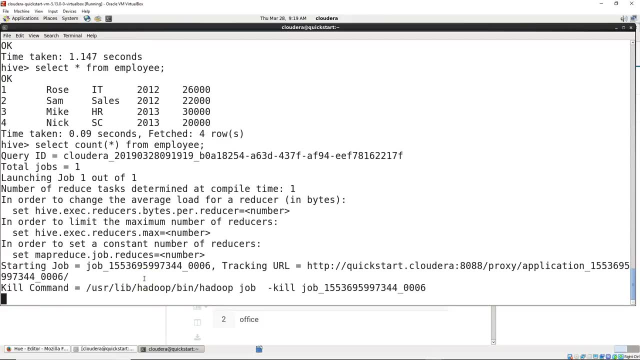 select options you can do. We're going to count Everything from employee. Now this is kind of interesting because the first one just pops up with a basic select because it doesn't need to go through the full map reduce phase. But when you 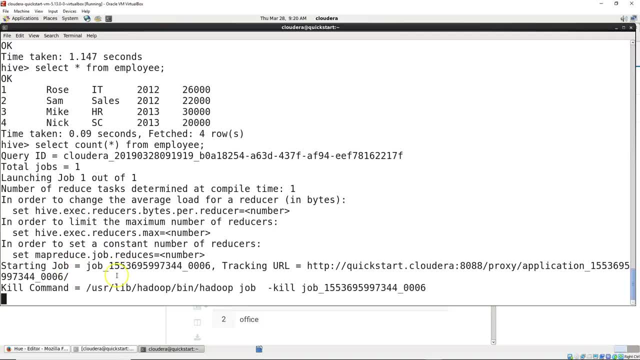 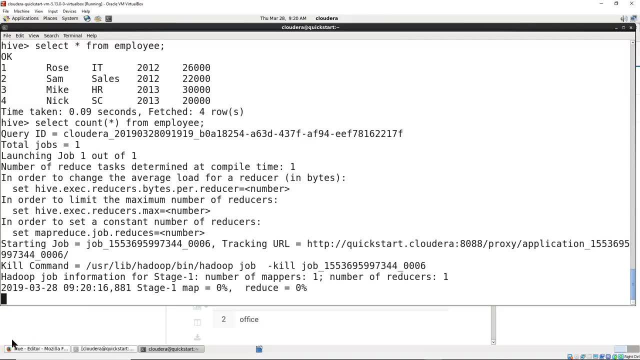 start doing a count, it does go through the full map, reduce setup in the Hive and Hadoop. And because I'm doing this demo on a single node- Cloudera virtual box on top of a Windows 10, all the benefits of running it on a cluster are gone And instead it's now going through all the 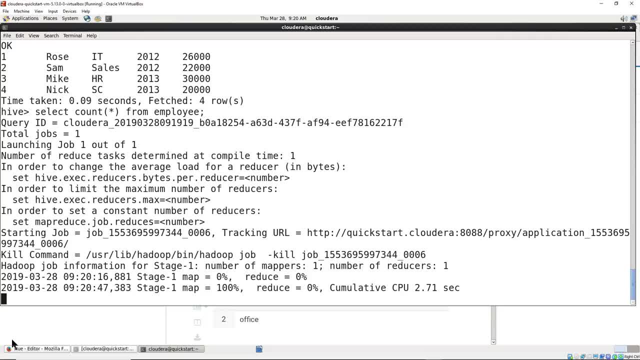 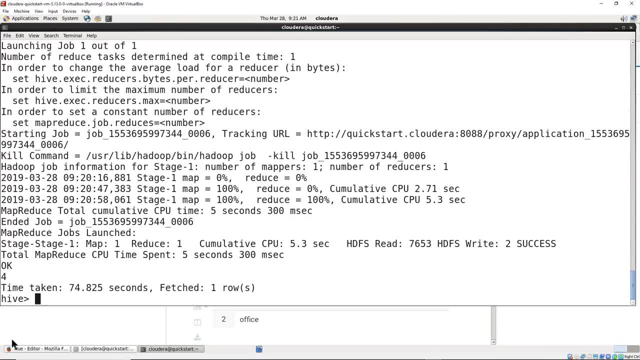 those added layers, So it takes longer to run. You know, like I said, when you do a single node, as I said earlier, it doesn't do any good as an actual distribution, because you're only running it on one computer And then you've added all these different layers to run it And we see it. 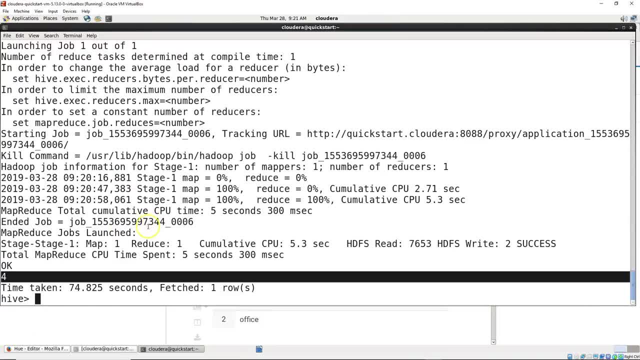 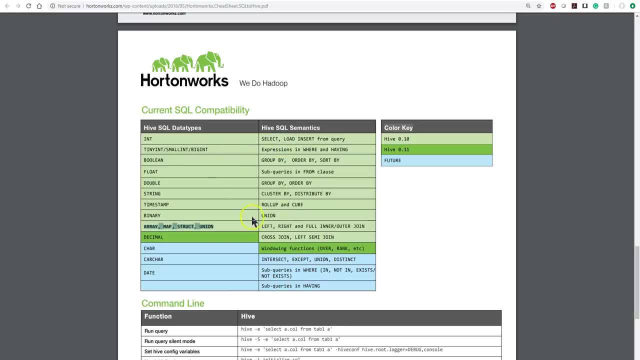 comes up with four And that's what we expect. We have four rows, we expect four at the end And if you remember from our cheat sheet which we brought up here from Horton's, it's a pretty good one. There's all these different commands we can do. We'll look at one more command where we do. 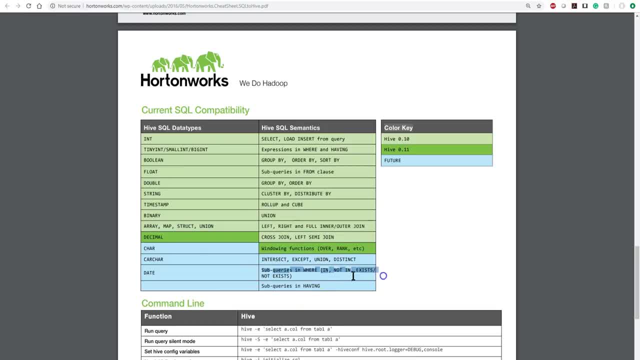 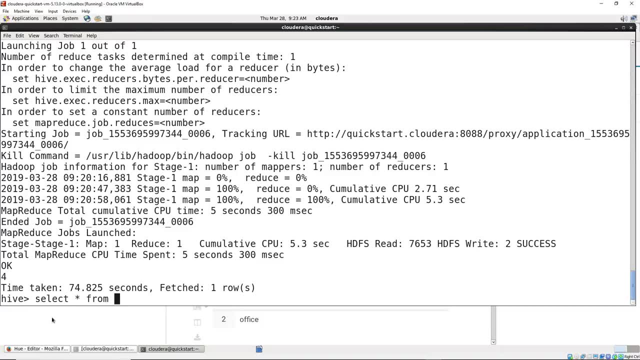 the what they call sub queries right down here, Because that's really common to do a lot of sub queries, And so we'll do select star or all different columns from employee. Now, if we weren't using the office database, it would look like this from: 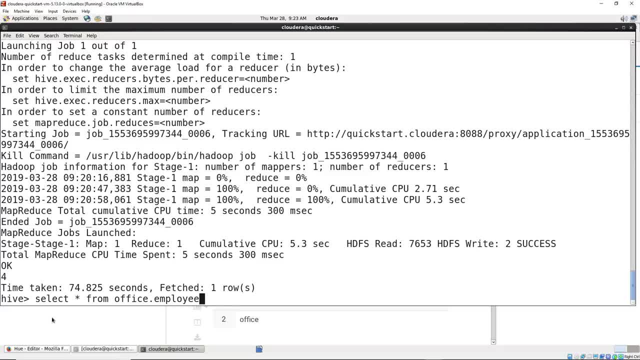 office dot employee And either one will work on this particular one because we have office set as a default on there. So from office employee and then the command where creates a subset And in this case we want to know where the salary is greater than the salary. And we're going to do 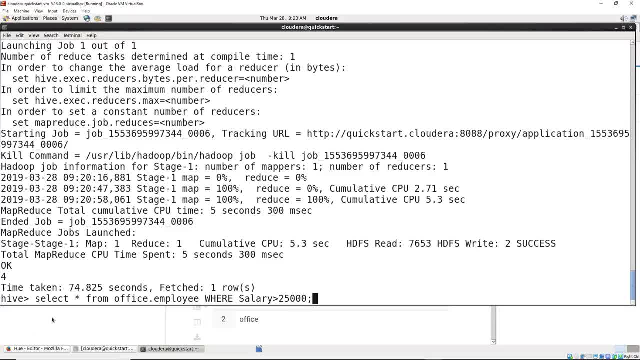 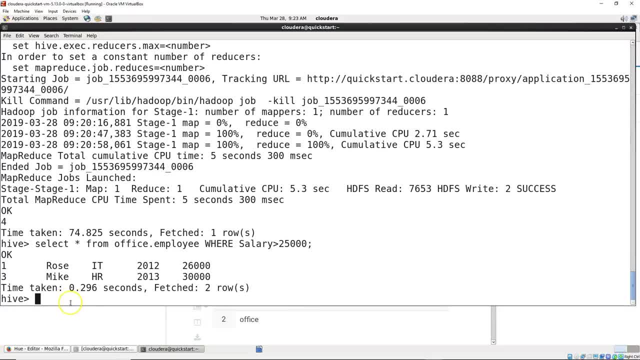 of course we end with our semicolon And if we run this query, you can see it pops up And there's our salaries of people, top earners. We have rows in IT and Mike and HR Kudos to them, Of course. 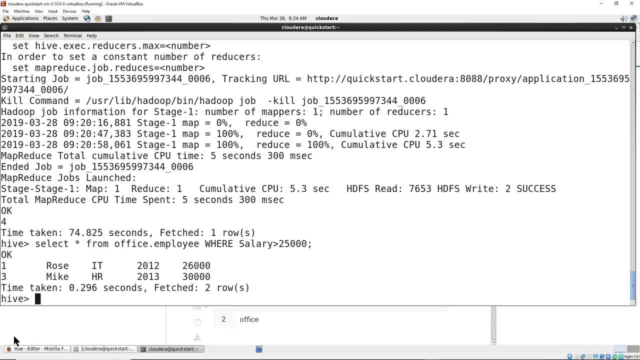 they're fictitional. I don't actually. we don't actually have a rows and a Mike in those positions, Or maybe we do. So finally, we want to go ahead and do: is we're done with this table Now, remember. 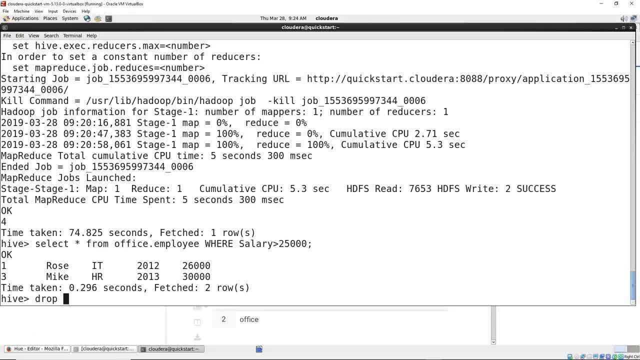 you're dealing with a data warehouse, So you usually don't do a lot of dropping of tables and databases, But we're going to go ahead and drop this table here Before we drop it. one more quick note is we can change it, So what we're going to do is we're going to alter table. office employee. 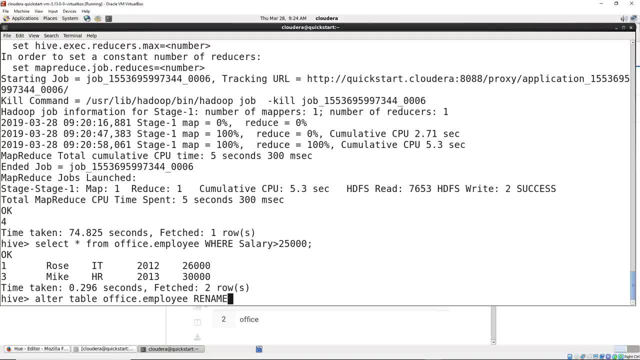 And we want to go ahead and rename it. There's some other commands you can do in here, But rename is pretty common And we're going to rename it to and it's going to stay in office And it turns out one of our shareholders really doesn't like the word employee. He wants employees plural, It's. 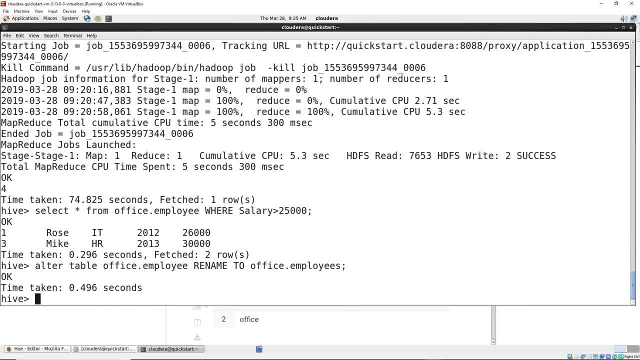 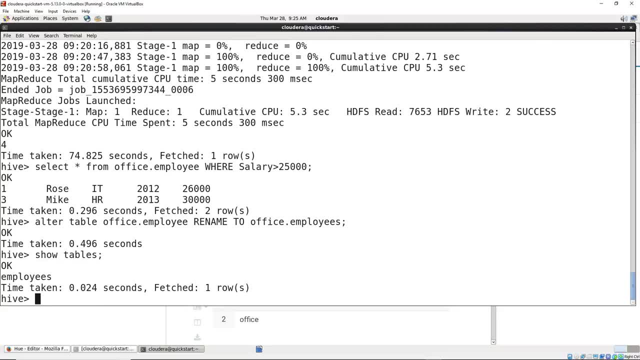 a big deal to him. So let's go ahead and change that name for the table. It's that easy because it's just changing the metadata on there. And now, if we do show tables, you'll see we now have employees, not employee. And then at this point maybe we're doing some house cleaning, because this 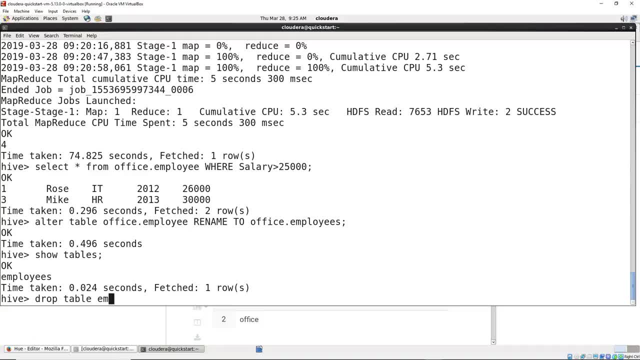 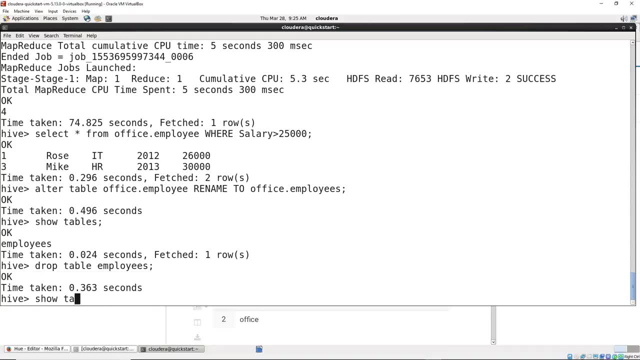 is all practice. So we're going to go ahead and drop table And we'll drop table employees because we changed the name in there. So if we did employee, just give us an error. And now if we do show tables, you'll see all the tables are gone. Now the next thing we want to go and take a look. 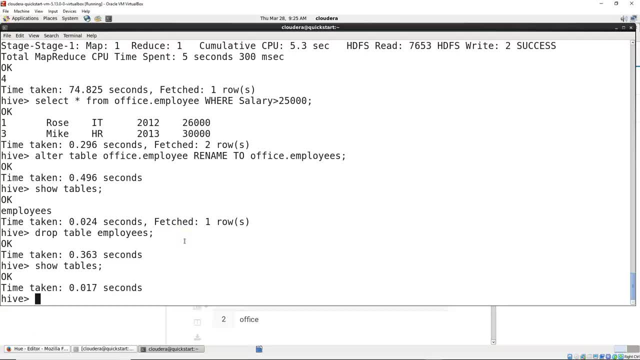 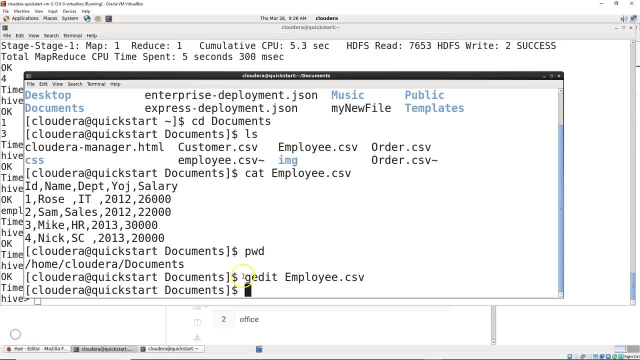 through the loading of data just real quick, because we're going to load two tables in here And let me just float back to our terminal window so we can see what those tables are that we're loading. And so up here we have a customer file and we have an order file. We want to go ahead. 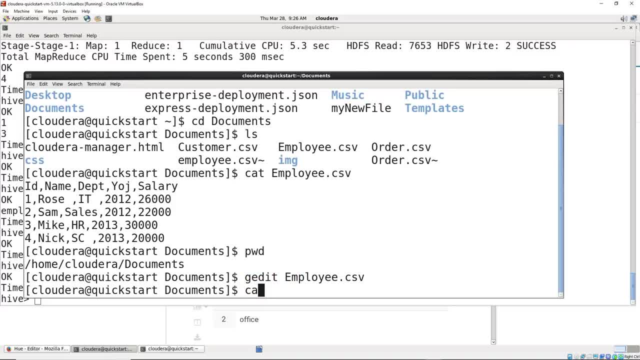 and put the customers and the orders into here. So those are the two we're doing, And, of course, it's always nice to see what you're working with. So let's do our cat customercsv. We could always do gedit, But we don't really need to edit these, We just want to take a look. 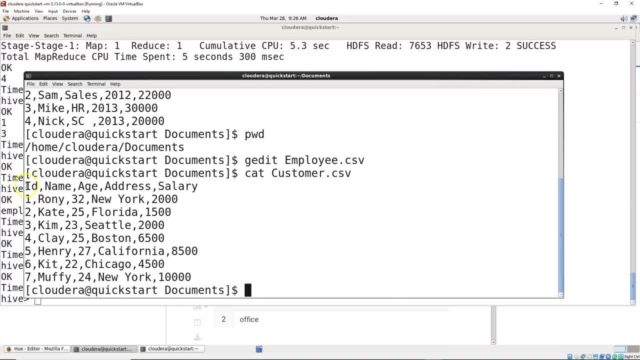 at the data in customer. And important in here is again we have a header, So we have to skip a line, comma separated. Nothing odd with the data. We have our schema which is integer, string, integer, string, integer. So you'd want to take that, note that down, or flip back and forth when 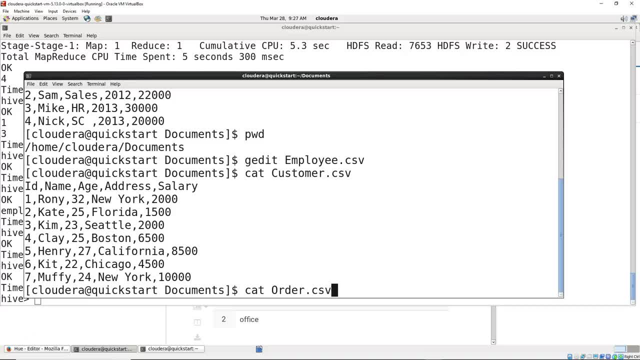 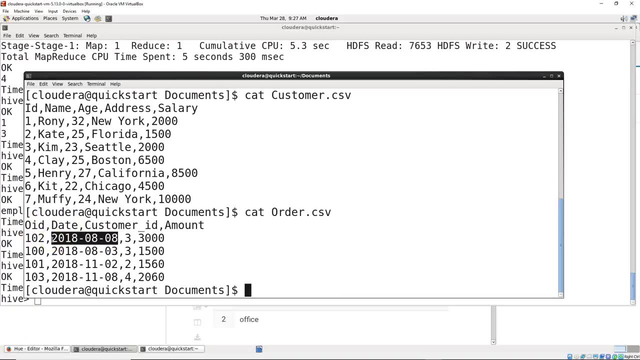 you're doing it. And then let's go ahead and do cat ordercsv And we can see we have oid, which I'm guessing is the order ID. We have a date. Oh, something new. We've done integers and strings. 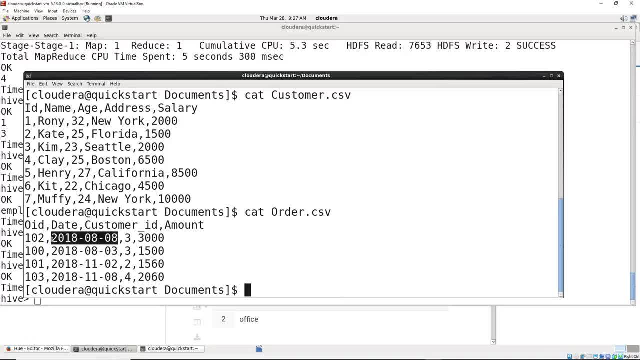 date When you're importing new and you never worked with the date. date's always one of the more trickier fields to port in, And that's true of just about any scripting language I've worked with. All of them have their own idea of how date's supposed to be formatted, what the default. 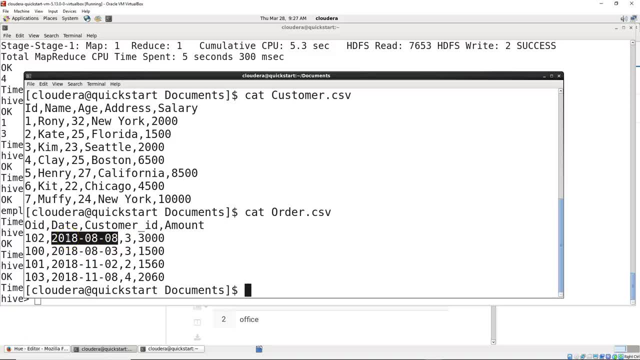 is This particular format, where it's year and it has all four digits dash month, two digits dash day, is the standard import for the hive. So you'll have to look up and see what the different formats are If you're going to do a different. 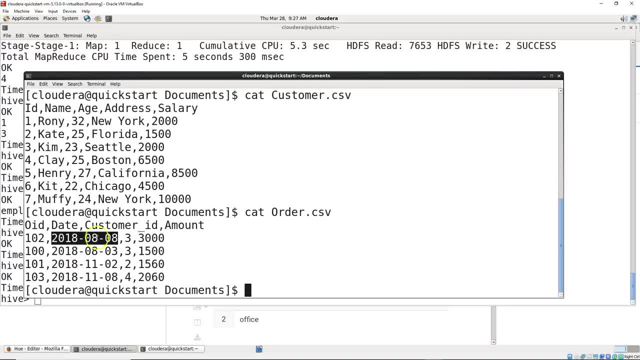 format in there coming in or you're not able to pre-process the data, But this would be a pre-processing of the data thing coming in. If you remember correctly from our etl, which is E- just in case you weren't able to hear me last time- ETL which stands for extract transform. 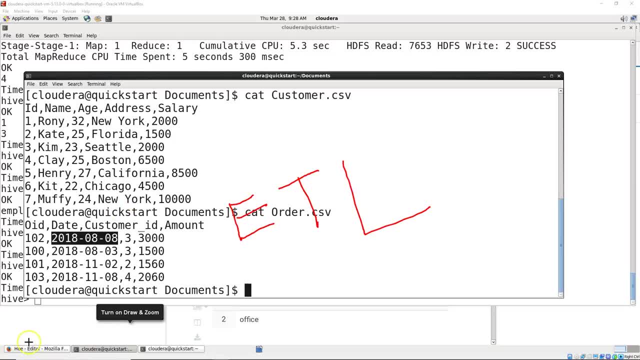 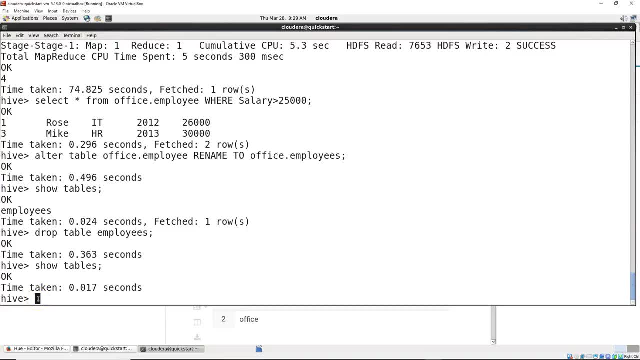 then load. So you want to make sure you're transforming this data before it gets into here, And so we're going to go ahead and bring both this data in here And really we're doing this so we can show you the basic join There is, if you remember, from our setup merge. 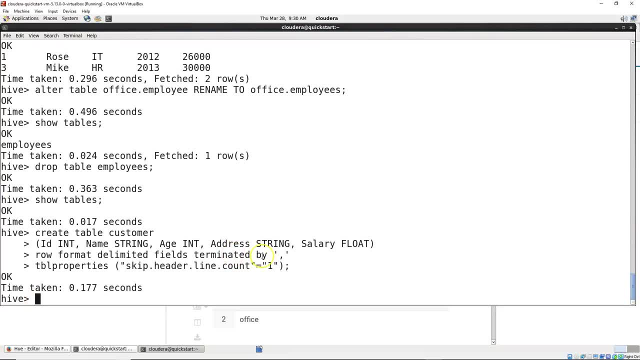 all kinds of different things you can do, But joining different data sets is so common, So it's really important to know how to do this. We need to go ahead and bring in these two data sets, And you can see where I just created a table: customer. Here's our schema: the integer name, age, address. 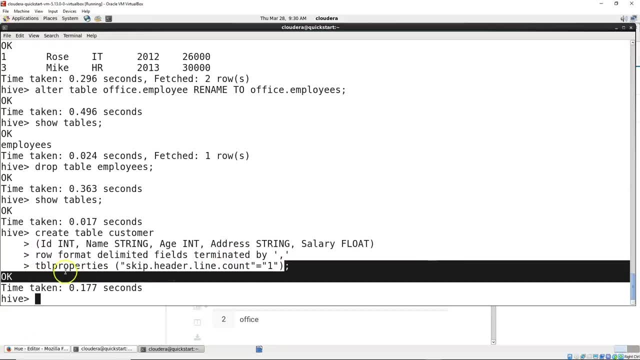 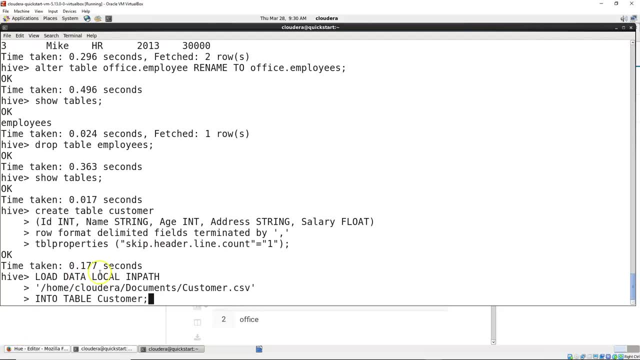 salary. Here's our, delimited by commas, and our table properties. where we skip a line, Well, let's go ahead and load the data first, And then we'll do that with our order, And let's go ahead and put that in here, And I've got it split into three lines so you can see it easily. We've got. 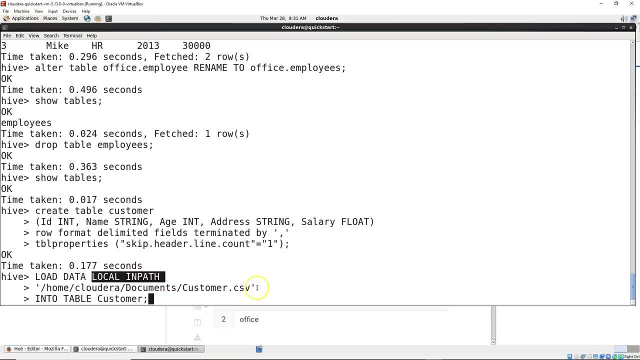 the path. So we know we're loading data, We know it's local And we have the path. Here's the complete path for oops. this is supposed to be order csv Grabbed the wrong one, Of course. 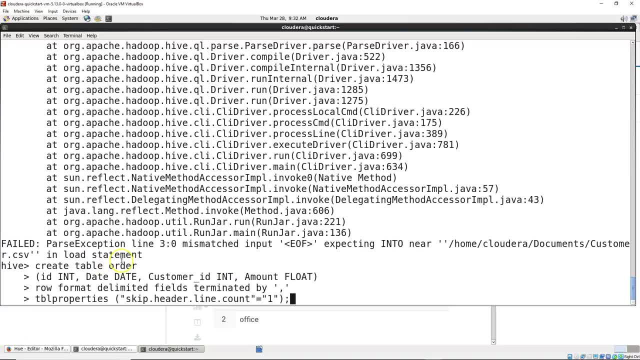 it's going to give me errors because you can't recreate the same table on there. And here we go, create table. Here's our integer date customer, the basic setup that we had coming in here for our schema: row format, commas, table properties. skip header line And then finally let's load the data. 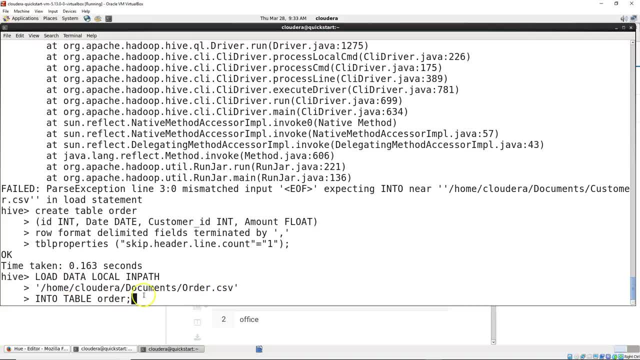 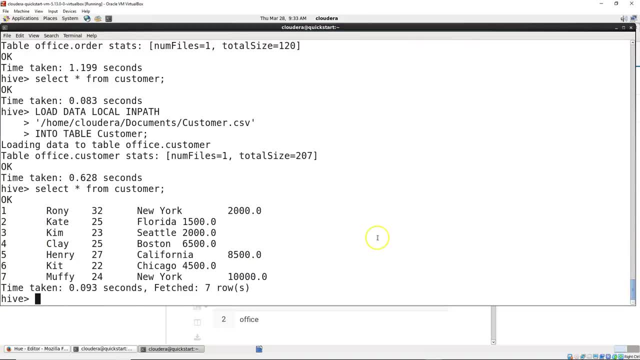 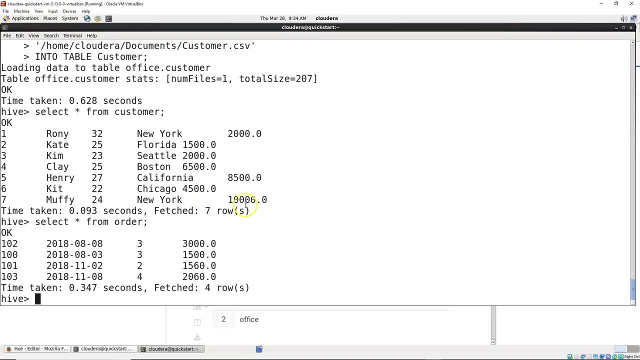 path home. Cloudera documents- ordercsv- into table order. Now, if we did everything right, we should be able to do select star from customer And you can see we have all seven customers. And then we can do select star from order And we have four orders. So this is just like a quick frame. 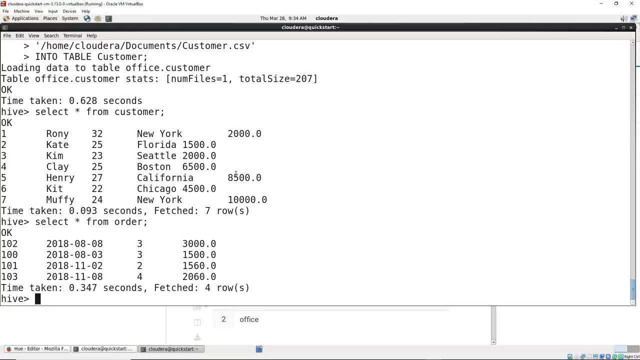 We have. you know, a lot of times when you have your customer databases in business, you have thousands of customers from years and years And some of them, you know, they move, they close names, all kinds of things happen. So what we want to do is we want to go ahead and find just 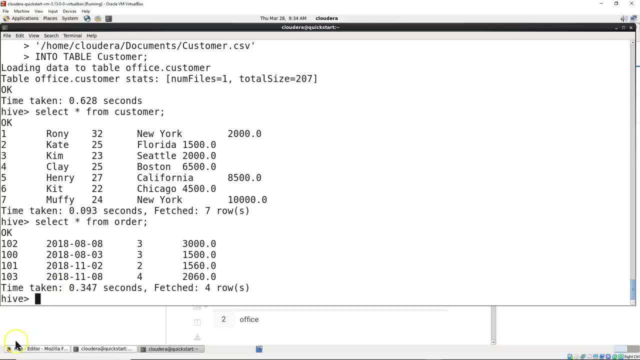 the information connected to these orders and who's connected to them. And so let's go ahead and do it's a select, because we're going to display information. So select, And this is kind of interesting- We're going to do cid And I'm going to define c as customer, as a customer table. 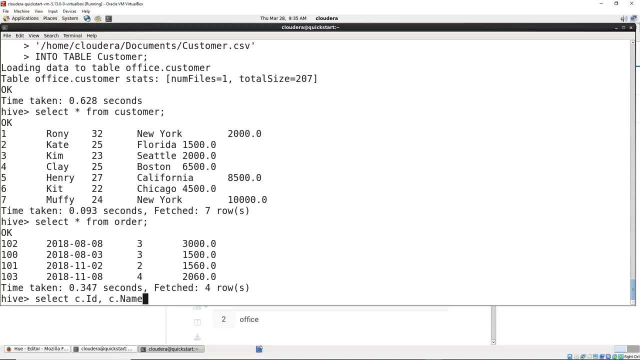 in just a minute. Then we're going to do cname And again we're going to define the c cage. So this means from the customer we want to know their ID, Their name, their age, And then you know. I'd also like to know the order amount. So let's do oamount. 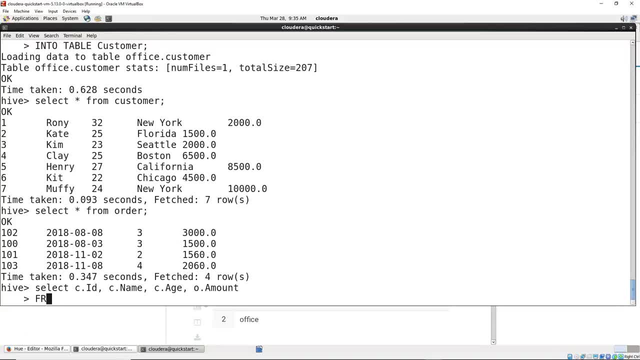 And then this is where we need to go ahead and define what we're doing, And I'll go ahead and capitalize from customer. So we're going to take the customer table in here and we're going to name it c. That's where the c comes from. So that's the customer table c And we want to join order as o. 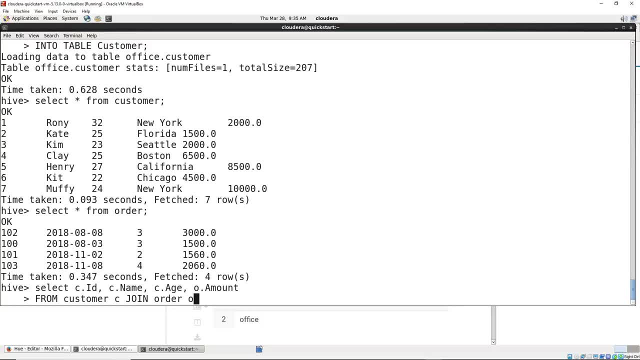 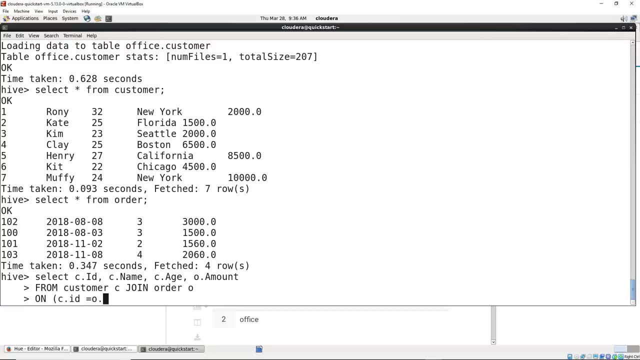 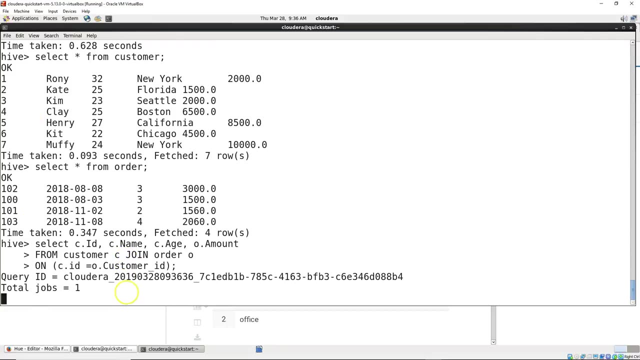 That's where our o comes from, So the oamount is what we're joining in there. And then we want to take the two tables. cid equals ocustomer underscore id. So now we know how they're joined. And now remember, we have seven customers in here, We have four orders And as it processes, we should. 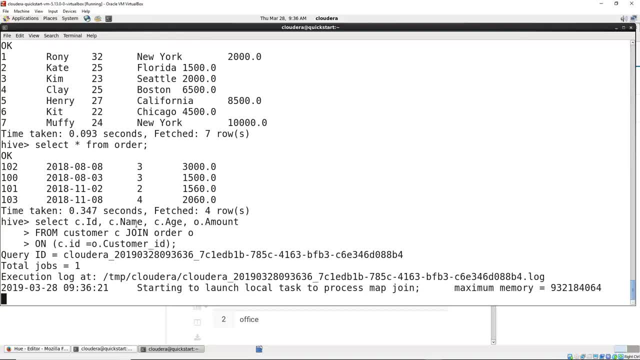 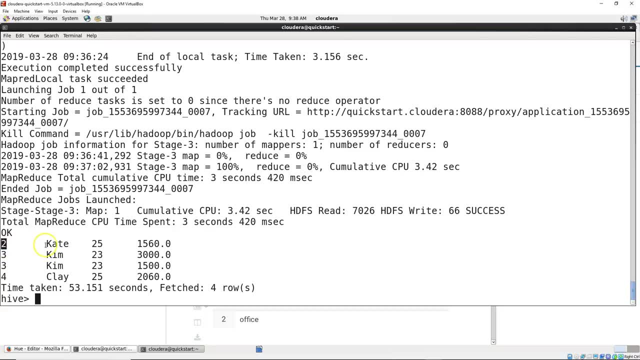 get a return of four different names joined together, And they're joined based on, of course, the orders on there And once we're done, we now have the order number, the person who made the order, their age and the amount of the order which came from the order number. So we're going to 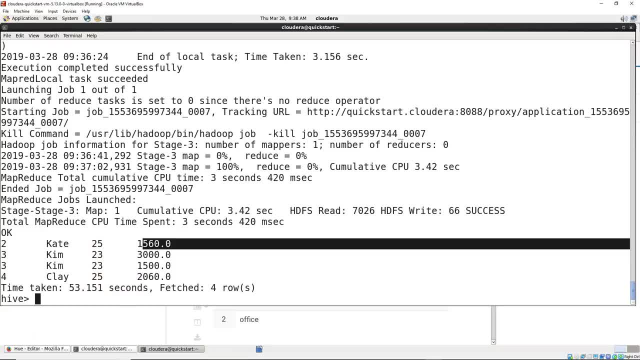 take the order table So you have your different information And you can see how the join works here. Very common use of tables and hql and sql. And let's do one more thing with our database And then I'll show you a couple other HIVE commands And let's go ahead and do a drop And we're going. 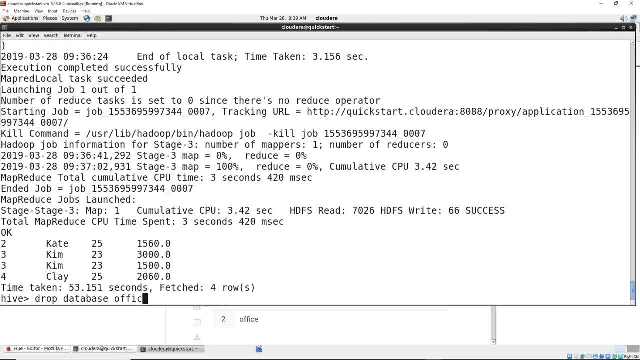 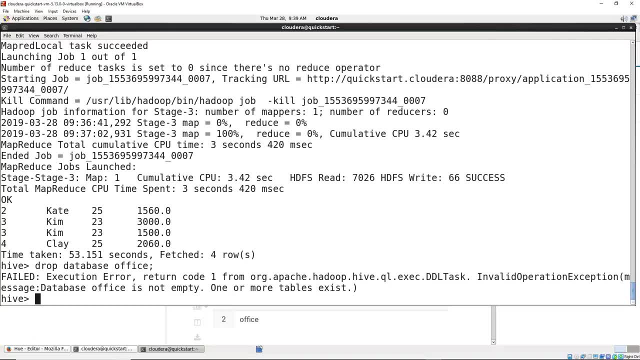 to drop database office And if you're looking at this and you remember from earlier, this will give me an error And let's just see what that looks like. It says: failed to execute exception. one or more tables Exist. So if you remember from before, you can't just drop a database unless you tell it to. 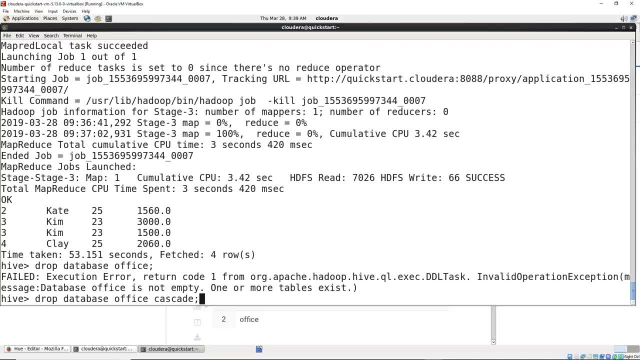 cascade. That lets it know. I don't care how many tables are in it, Let's get rid of it. And in Hadoop, since it's a warehouse, a data warehouse, you usually don't do a lot of dropping, Maybe at the 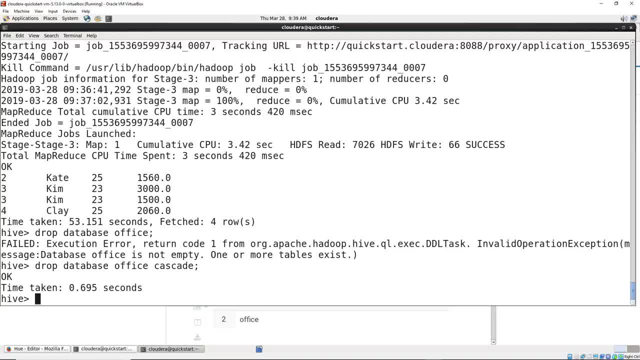 beginning, when you're developing the schemas and you realize you messed up. you might drop some stuff. But down the road you're really just adding commodity machines to take up so you can store more stuff on it. So you usually don't do a lot of database dropping And some other fun commands. 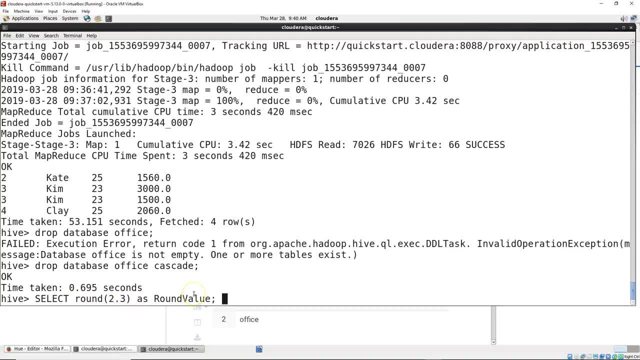 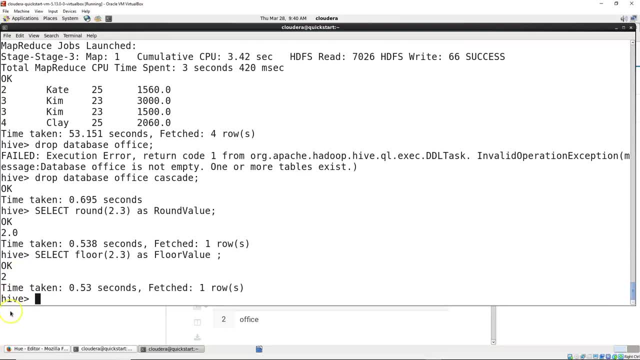 to know is you can do select round 2.3 as round value. You can do a round off in hive. We can do as floor value, which is going to give us a two. So it turns it into an integer versus a float It. 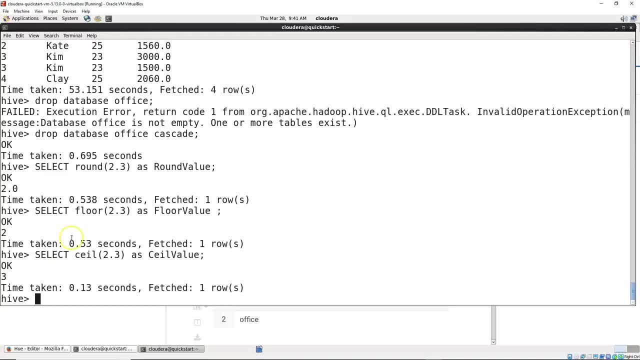 goes down, basically truncates it, but it goes down And we can also do ceiling, which is going to round it up. So we're looking for the next integer. above There's a few commands we didn't show in here because we're on a single node As an admin, to help speediate the process. 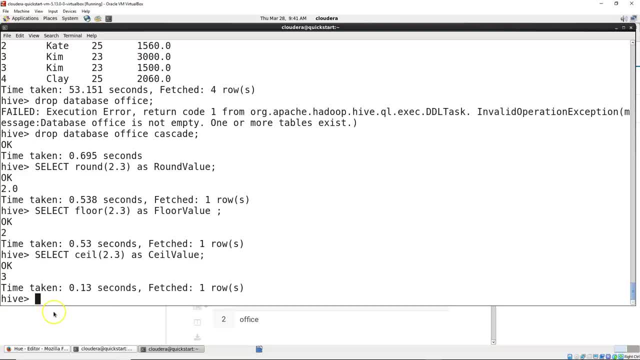 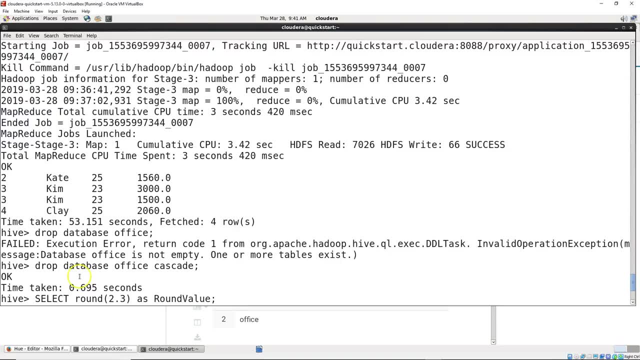 you usually add in partitions for the data in buckets. You can't do that on a single node because when you add a partition, it partitions it across separate nodes. But beyond that you can see that it's very straightforward. We have SQL coming in And all your basic queries. 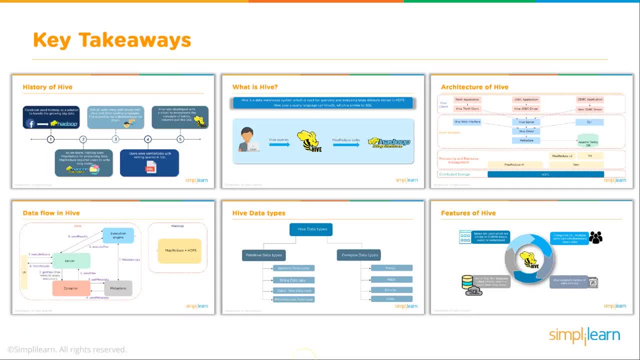 that are in SQL are very similar to HQL Key takeaways. So we took a look at the history of Hive and how it evolved from the Hadoop file system to an HQL similar to SQL layer on top of Hadoop, with the full meta store and all that information connected to the Hadoop file system. 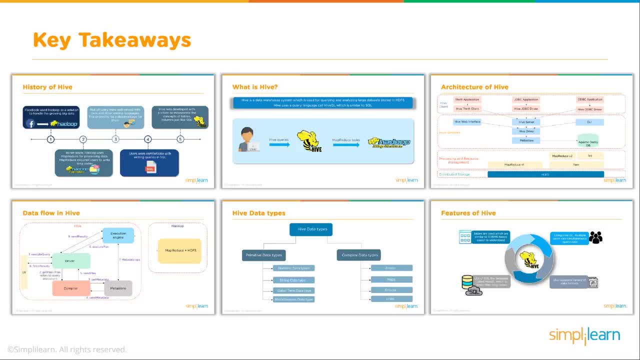 That way you can easily scale it up and still have underneath the Hadoop setup while still having the SQL query language available. We looked at what is Hive And we looked at the Hive queries going in through the MapReduce into the Hadoop MapReduce system. We dug a little deeper to look. 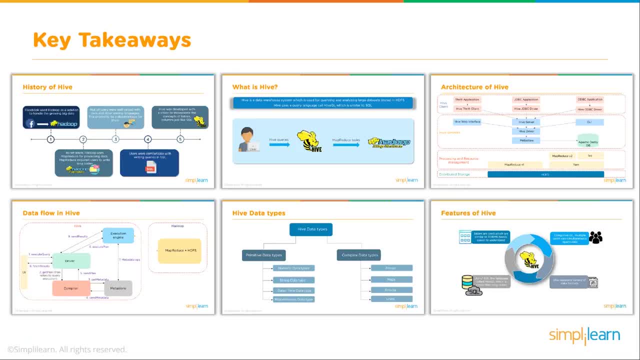 at the architecture of Hive and all the different pieces and how they fit together, including the fact that it has the Hive client and you have your Thrift application And your JDBC applications and your ODBC applications. We have the Hive web interface, which we looked at in a demo, along with the CLI, which your client direct interface. 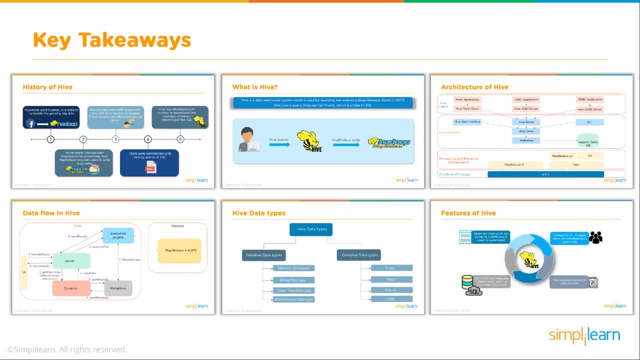 which we use for most of the demo. And again, this is: how do you get these commands into Hive? And if you're using the Hive web interface is great, for maybe your shareholders you're working with and some of them are not technically literate, or even if they are, you know.